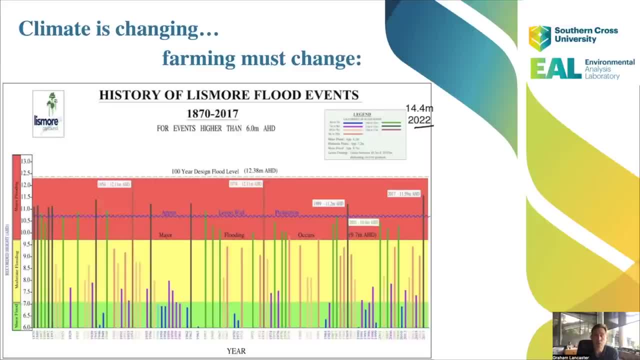 around the world. Just in Lismore we just had two weeks ago our biggest flood on record, but not just on record but broke the records. So the whole town or the whole city went under a couple of billion dollars damage. You can see here on this graph right back to 1870,. 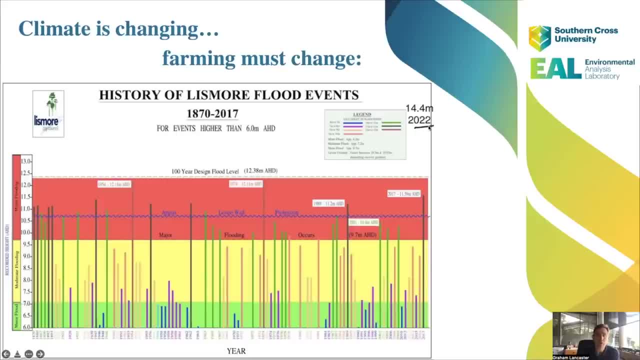 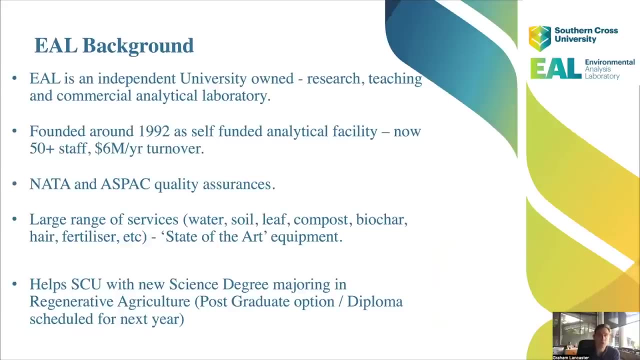 14.4 meters is where we got to over the right here in March 22, and it's just not even on the scale of the maps. And that's what's going to happen all around the world. So just expect the unexpected these days. On to my presentation. a little bit about EAL. EAL is an independent university-owned. 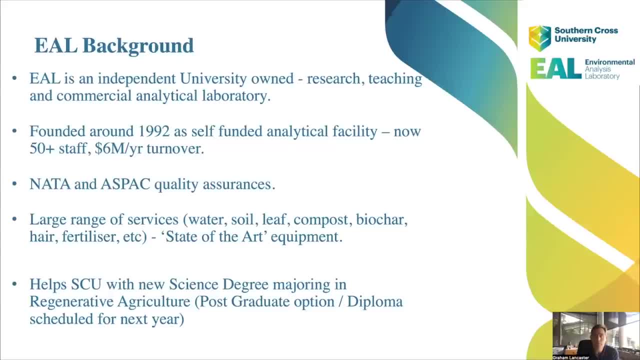 research, teaching and commercial analytic laboratory. We're stationed here in Lismore, up on the hill, luckily- but it's an independent university-owned research, teaching and commercial analytical laboratory. We're stationed here in Lismore, up on the hill, luckily. 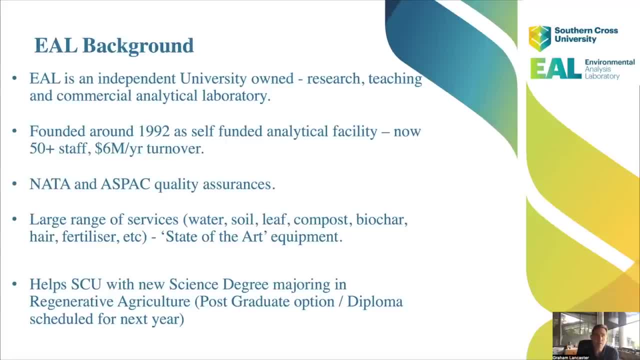 but it's an independent university-owned research, teaching and commercial analytic laboratory. We're stationed here in Lismore, up on the hill, luckily, but it's an independent university-owned research, teaching and commercial analytic laboratory. We're stationed here in Lismore. 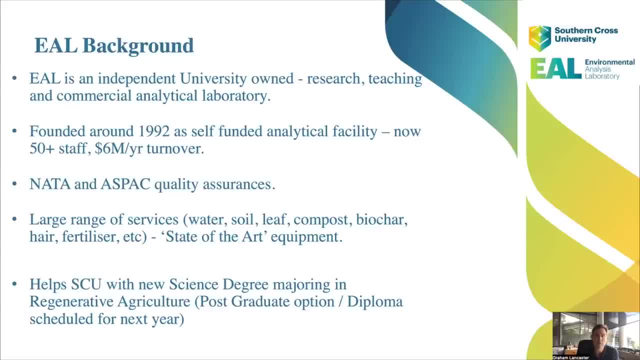 the studio is visitable through the skyline and you can see the university and the lab in the background there. I founded it as a student- undergrad student in environmental science in about 92, and we've always been a self-funded facility, So the university gets a lot out of us. 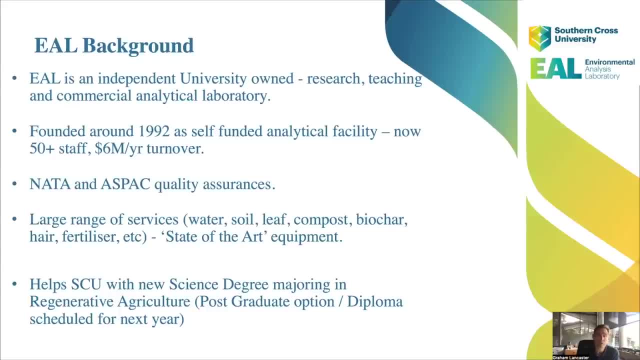 and we get a lot from the university. We now have well over 50 staff and we're turning over $6 million a year, So a reasonable-size laboratory. We're NARTA and ASPAC quality assurance- NARTA's National Association of Testing Authorities and ASPAC's Australia's National Association of Testing. 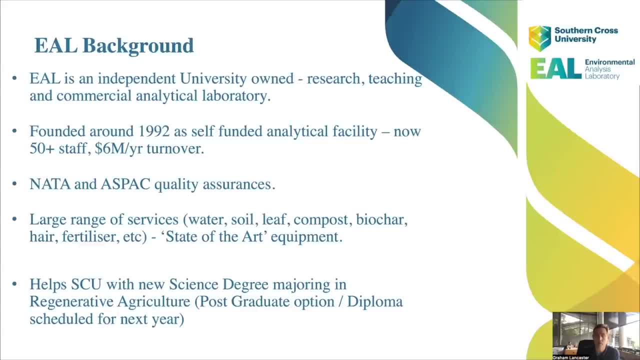 Authorities and ASPAC's Australian Soil Plant Analysis Council. So we concentrate on getting the right results, which is so important for labs around the world. We have a large range of services. I always like to be a one-stop shop. So from water to soil, to leaf to compost. 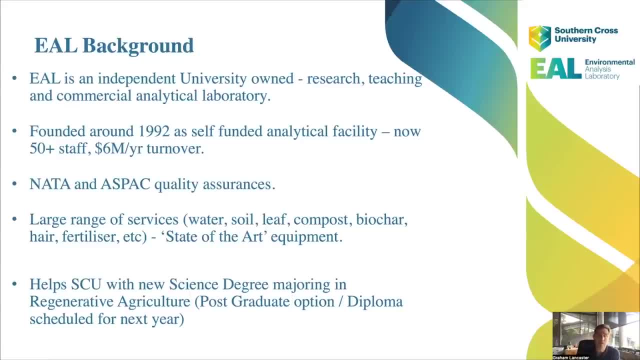 to biochar, to human hair testing and animal hair testing to fertiliser. We have state of the art equipment, which is about being in a university but also bringing in the money to afford that equipment. We work with Southern Cross Uni on a new science degree majoring. 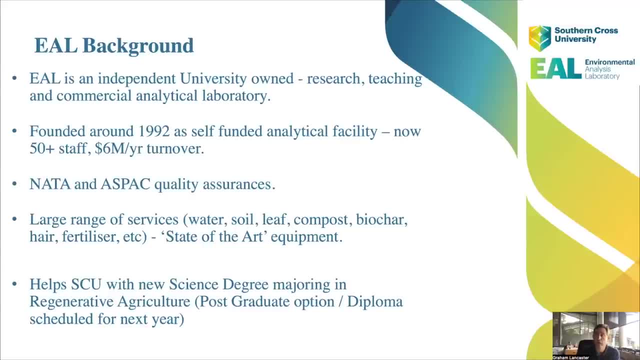 in regenerative agriculture, which opened now a year and a half ago and been hugely successful with hundreds of students going through that program. We now have a post-grad option and a diploma scheduled next year, which is all fantastic to see We've been involved with. 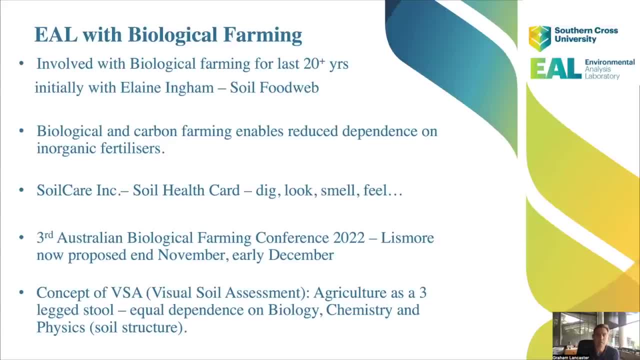 biological farming. We've been involved with organic farming. We've been involved with organic farming now for well over 20 years. with Elaine Ingham and Soil Food Web, We ran a course maybe 10 years ago now. for 10 years that was hugely successful- a two-week course. 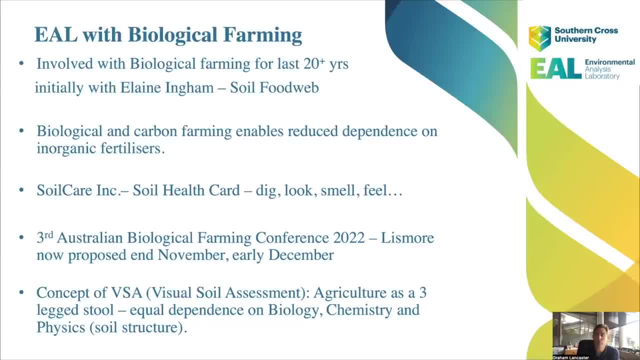 Biological and carbon farming enables reduced dependence on inorganic fertilisers. I know Elaine likes to push no inorganic fertilisers and if you're a fully successful biological farmer, yes, I think that can be achievable with a really good compost Soil care. we work a lot with our local Soil Care and Soil Health Card is something that 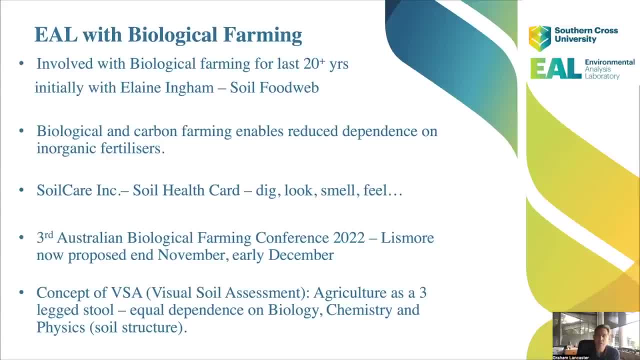 they produce and freely available on the web. where you dig, look, feel, smell, do everything with your soil to really know your soils, and I think that's a really important aspect of understanding your farm and your farming. We are also organising the third Australian. Biological Farming Conference. this year. We are also organising the third Australian Biological Farming Conference this year. We have a number of different groups on the website at the website. I think it's a great way to get in touch with your community. We've been involved. 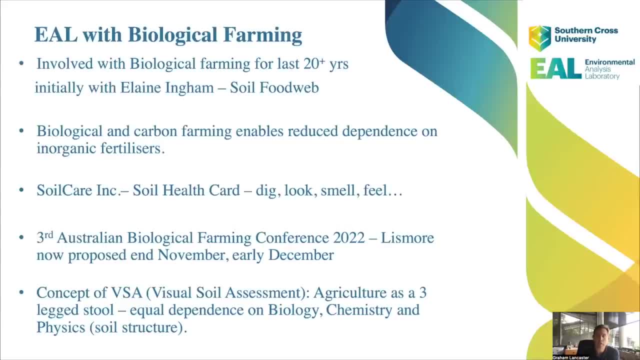 it's going to be pushed back a bit now, proposed for the end of November to early December, and also- I love that- just the simple concept of visual soil assessment. this is produced around Australia, but I'm sure around the world as well, where agriculture is a three-legged stool. you 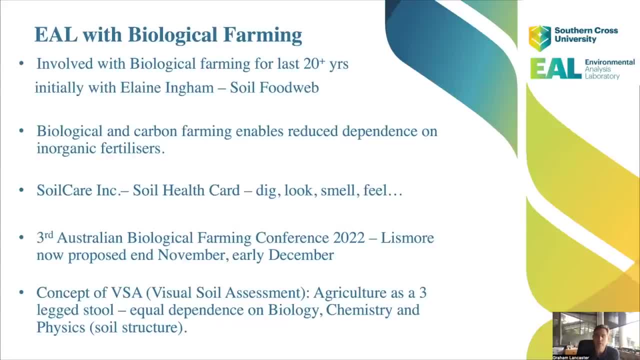 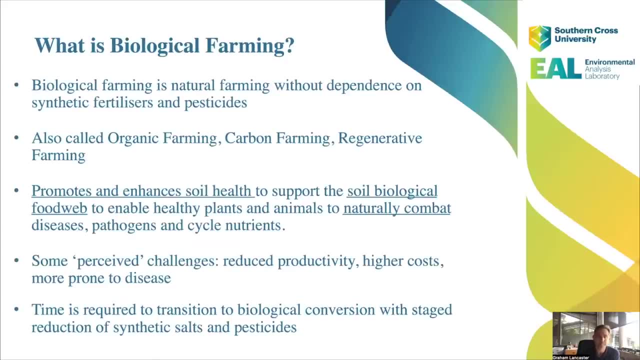 really need the biology, you need the chemistry and you need the physics. the soil structure and all these aspects are so important and I'll talk a lot about these now. biological farming is natural farming without dependence on synthetic fertilizer and pesticides. that's just how simple it is. we call it organic farming, carbon farming, regenerative. 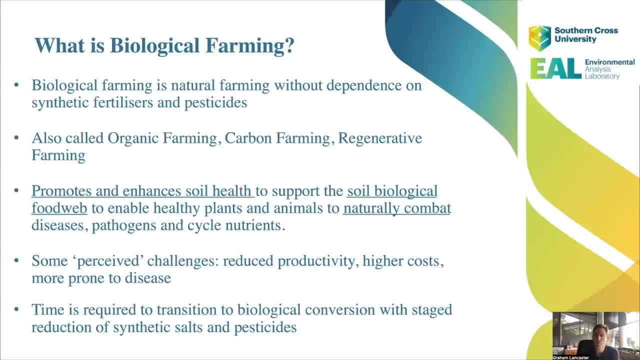 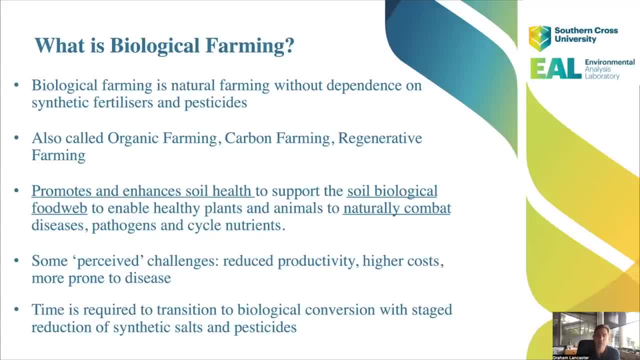 plants and animals and to naturally compact diseases, pathogens and cycle nutrients. some perceived challenges reduce productivity, higher costs, more prone to disease. I think it's all opposite. if you're a successful biological farmer, you're increasing your productivity, you're reducing your costs, because fertilizer costs these days are going up and up. 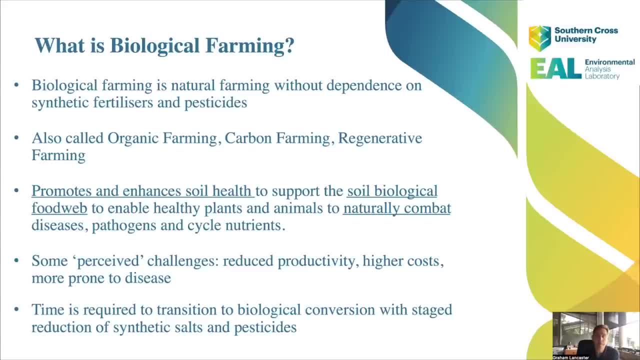 and pesticide costs are ridiculous but- and you should be less prone to disease because your crops should be so much healthier- time is required for transition. I don't think this can happen overnight. you've really got to do stage reduction, I believe, of synthetic fertilizer, salts and pesticides, and I think that's important. I don't want to see anyone going. 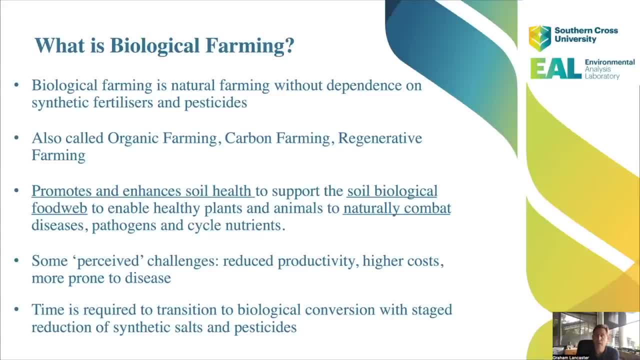 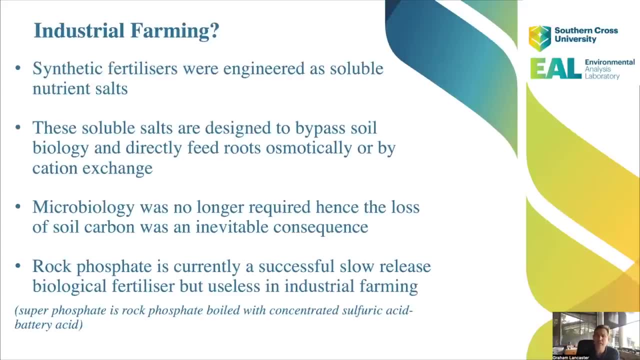 backwards. so really just reduction is a first goal, and then the elimination of these additives. industrial farming- so what is industrial farming? it's, it's really what it takes to have a Онлайн 産業 treball. So what is industrial farming? 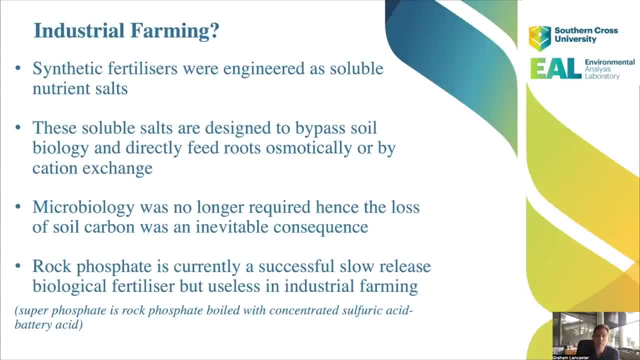 It's really what it takes to have a운ail How to produce vegetables on your own. really, what farming has become worldwide? its synthetic fertilizers were engineered as soluble nutrient salts. these soluble salts are designed- whether we design it that way or not- to bypass. 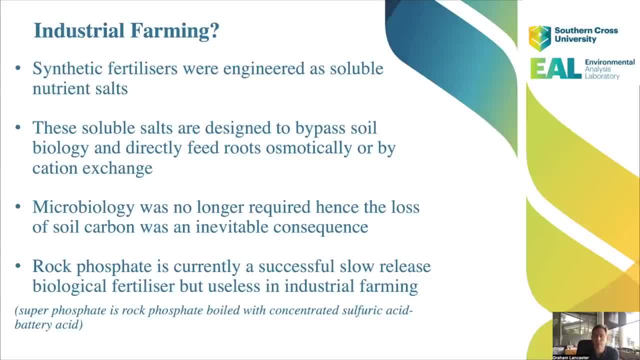 soil biology and directly feed the roots osmotically and chemically and all the rest by cation exchange. microbiology was no longer required and actually doesn't exist in a lot of industrial type farms where high pesticide use has occurred and hence the soil carbon loss has been astronomical, and without soil carbon in your soil, well, you've got dirt and 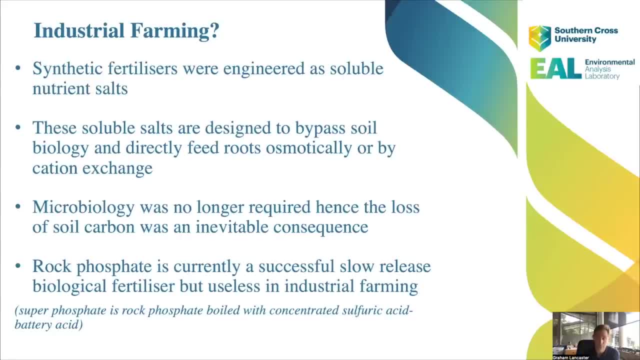 we don't really want dirt, we want proper soils, we want a living ecosystem. rock phosphate is currently- and there's a lot of other natural fertilizer products like this- a successful slow release biological fertilizer, but useless in industrial farming because in a farming system where you don't have soil biology, nothing releases those nutrients it. 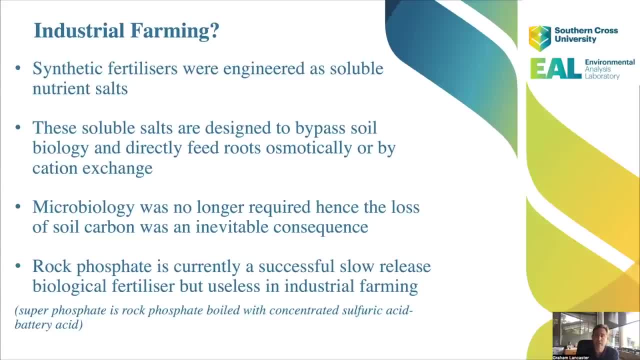 just sits in the soil, a bit like compost. if you add compost to a a non-biological farm, it'll sit on the surface or sit in the soil and just not decompose because you haven't got the soil biology just out of information. super phosphate you. you wonder how that's made? it's made by having rock. 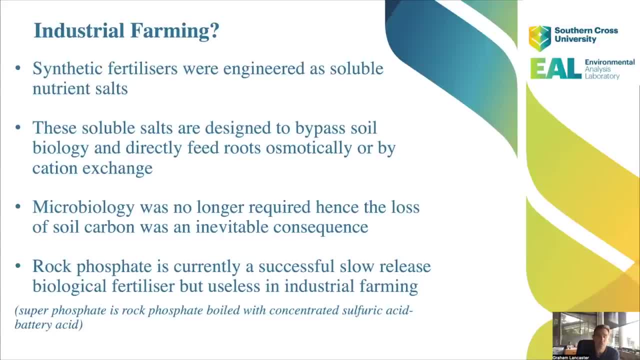 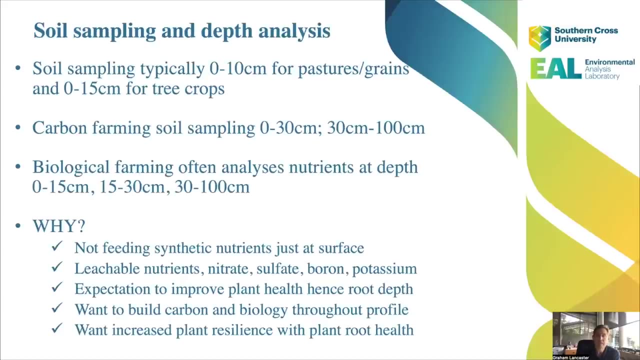 phosphate boiled with concentrated sulfuric acid, which is battery acid, and that's how they make super phosphate all different forms and it's just purely chemically made and once again it's biologic, bypassing biological processes, soil sampling and depth analysis. look, soil sampling is typically naught to 10 centimeters. 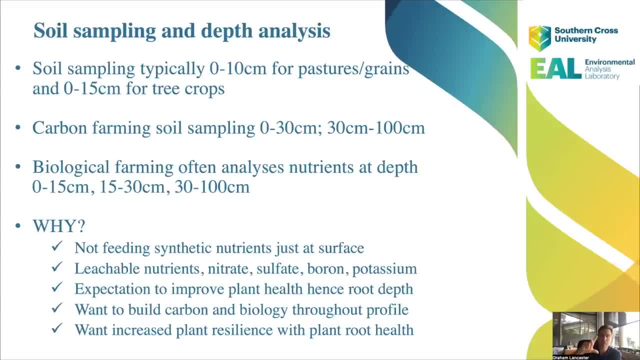 which is just a small amount, and then for 15 centimeters for tree crops. why is that the case? well, i think because, yeah, we've just historically fed nutrients in the top layer of soil. carbon farm in the top layer of soil. carbon farming in australia and, i'm sure, worldwide will. 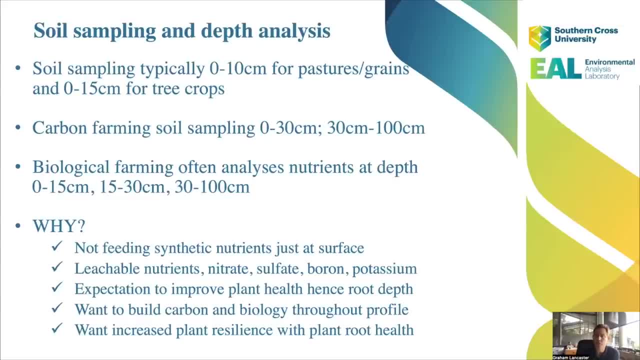 follow. the same sort of example is naught to 30 centimeters and 30 to 100 centimeters. so you could ask the question: why is that the case? well, i believe that's the case purely because with biological processes, we are activating carbon down the soil profile. 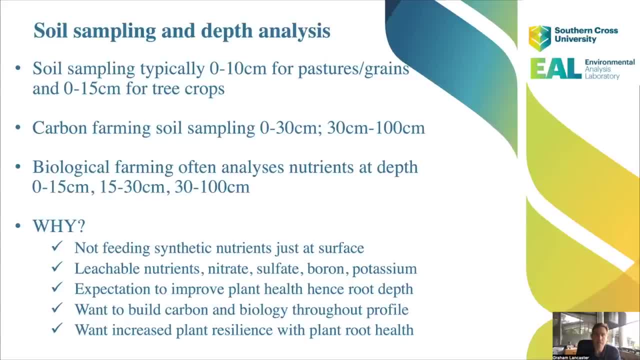 we're activating the roots and all the rest. so, um, if we were not activating the soil, biology- and that's how we get the increases in carbon, then we wouldn't need to go to these sort of deaths. but we've had some amazing research here by christine jones and others where they've shown huge 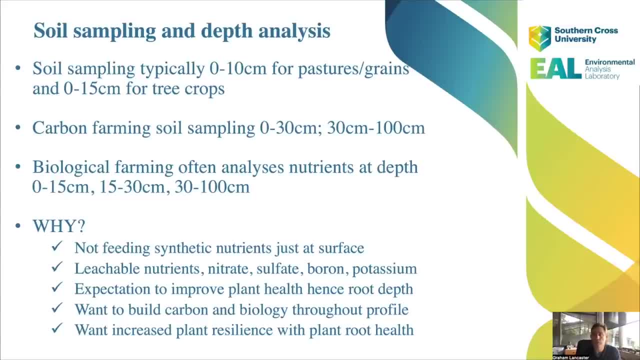 increases in carbon down to that 30 centimeters to 100 centimeters depth in your soil profile. but note this: all depends on your soil type. some soil types it's not as successful and it's really dependent on your region and often in biological farming we encourage testing the nutrients at depth. 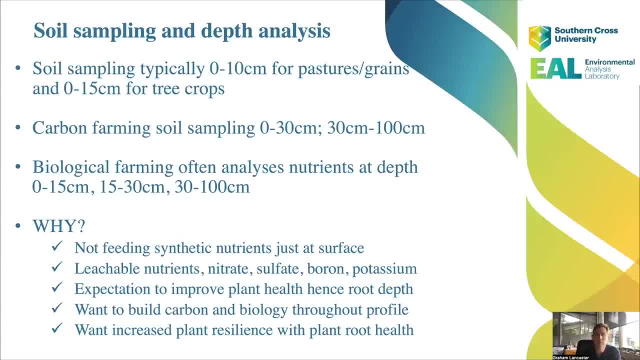 in some sort of profile naught to 15 centimeters, 15 to 30 centimeters and 30 to 100 centimeters. you might only do this once in once in the life of your farm, but just to get an idea on what your nutrient is, write down your profile. so why do this sort of depth analysis? because we're not just 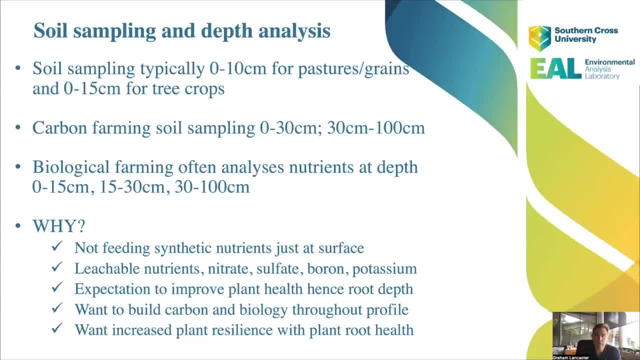 feeding synthetic nutrients. at the surface leachable nutrients like nitrate, sulfate, boron and potassium go down your profile and you really want your roots to go down that way as well. expectation to improve plant health. health enhance root depth. want to build carbon and biology throughout the profile. 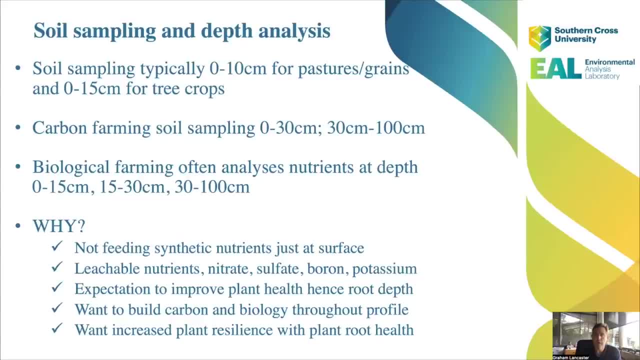 and you want to increase plant resilience with plant root health. so you think about when we get an extra out. if you've got your roots going down half meter or a meter and not just sitting on that surface, think of the water access those roots have. it's massively different, as you can understand. 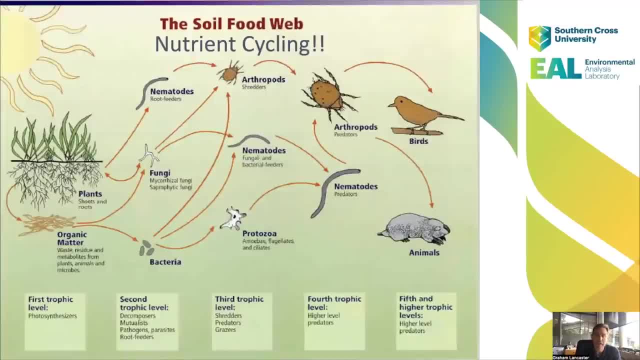 now, i know you know these, these diagrams, and this is one by elaine um soil. food web promotes it. it's such a simple diagram. all i see here, with outputting my biology hat on, is nutrient cycling. every pathway here is a change in nutrients, a consumption of nutrients. 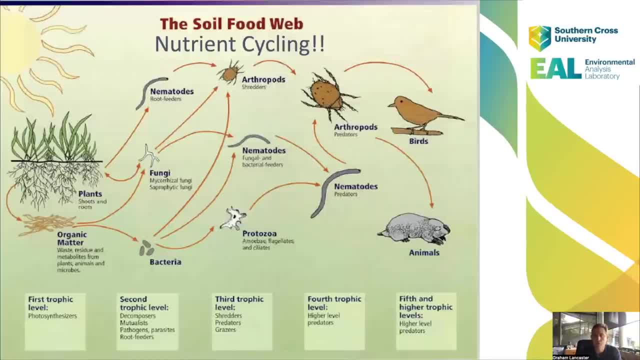 and a release of nutrients, a binding of nutrients and release of nutrients. so you've got to start with this organic matter and think about organic matter. it's, it's the tiny bits you can't see in the soil, and i'll talk a little bit about the testing of that in a moment. 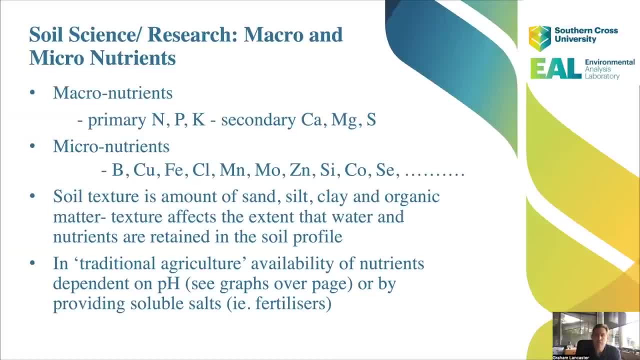 so soil science, research, macro micro nutrients, really in industrial farming, npk, that's all they seem to know about. but then, just out of interest, they like to add other nutrients because they like to think it's not just about npk. so they add calcium, magnesium, sulfur as your macro nutrients. 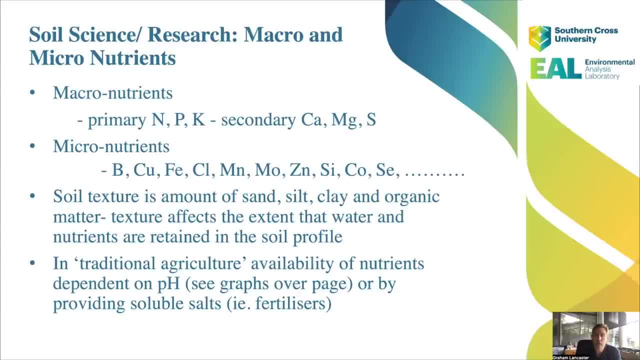 and then your micronutrients by boron, copper, iron, chlorine- which is probably less important, more than of a toxic element- manganese, molybdenum, zinc, silicon, cobalt, selenium, and it goes on and on. soil texture is so important. you've got to understand your soil texture for your 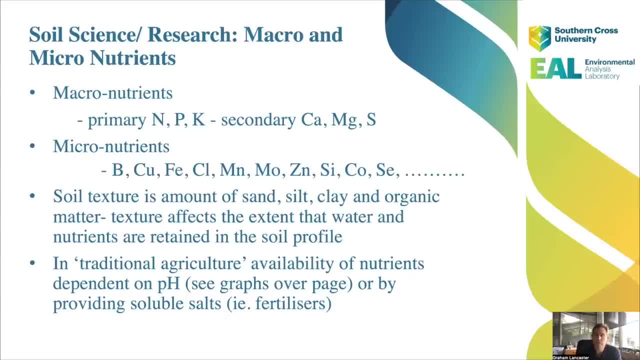 farm or your system or your region. it's the amount of sand, silt, clay, organic matter. texture affects the extent the water and nutrients are retained in the soil profile in traditional agriculture um available nutrients, or traditional, as i say, industrial agriculture um availability of nutrients dependent on ph. so i'll have some graph on that. 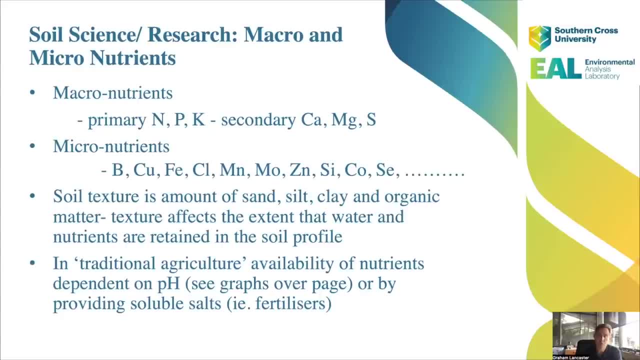 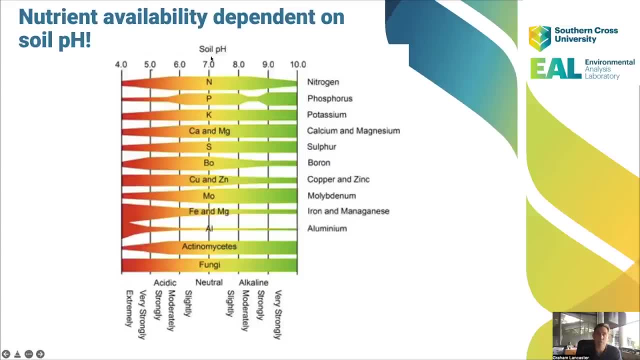 or by providing soluble salts um fertilizers. these sort of graphs a lot of the agronomists run around with and say you've got to get your ph at seven because that's when you get your maximum availability of nutrients. that's funny how they put um some of your microbes in here. 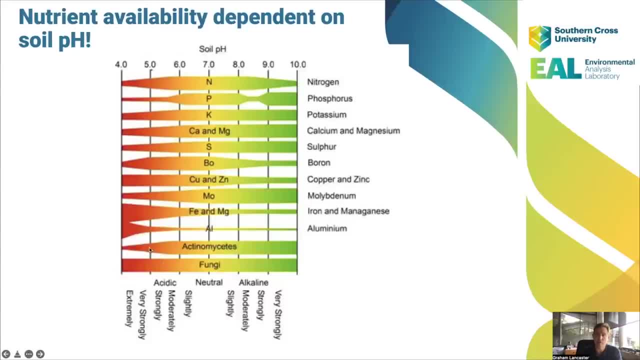 um, but what this has shown at the lower levels- um ph levels, ph5 and below- then your microbes aren't even liking it. we don't need to look at this at all in biological agriculture, because i've seen so many farms- biological farms- that are very comfortable at a water ph of about five to. 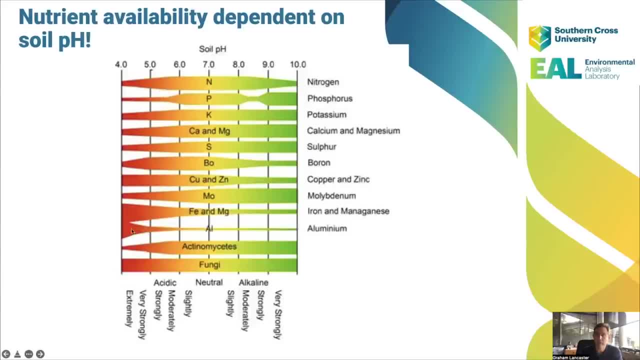 five and a half. it's only when you get below that that you start getting this aluminium and iron toxicity, and that is a real problem. um, and unless you've got a hugely successful biological system, you really want to keep your ph above um the five to five and a half. however, note it's not just. 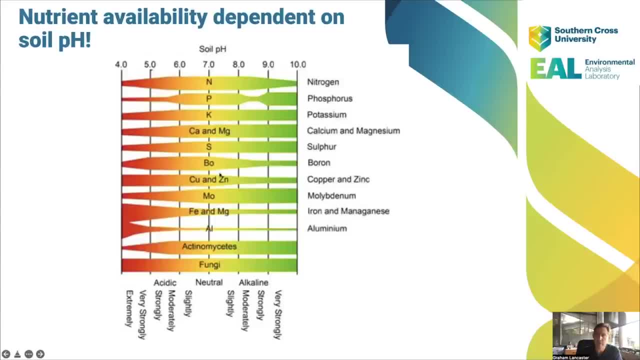 with lime. organic matter is actually a fantastic buffer of ph in soil, so it's not just lime you're using, but if you have a good organic carbon organic matter content in your soil, you're bringing up that ph by itself. so have a good compost source and it's not just lime but you. 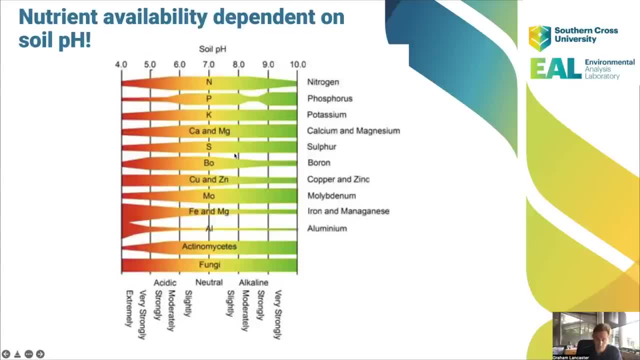 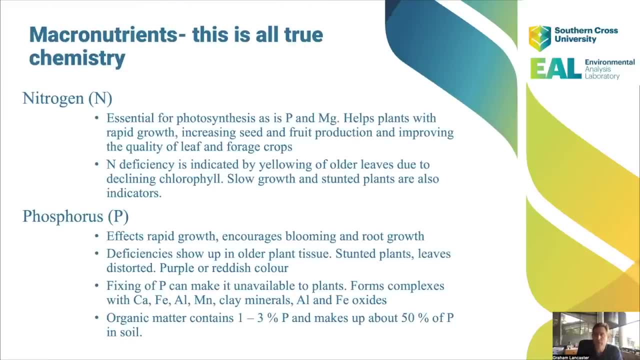 do want to look at this to some extent, but really nothing like you if you're doing this industrial farming now. these are all things that have been learned in soil chemistry. i'm not going to go through them in a big way, but it is true these elements all play a major part in our soil. 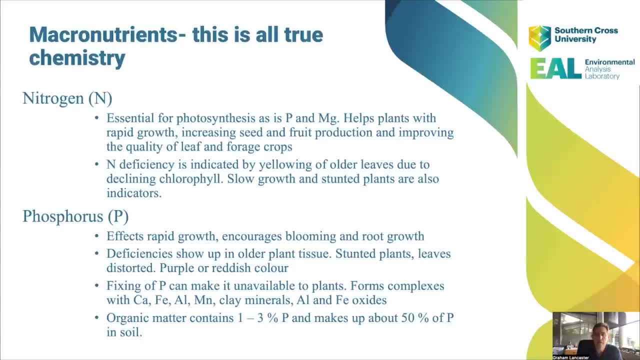 biology and our soil growth. plant growth um this example. they're nice and essential for photosynthesis, as is p in magnesium, phosphorus and magnesium. health plants with rapid plants with rapid growth, increased seed and fruit production, improving quality of leaf and forage. nitrogen deficiency is indicated by yellowing of olive leaves due to. 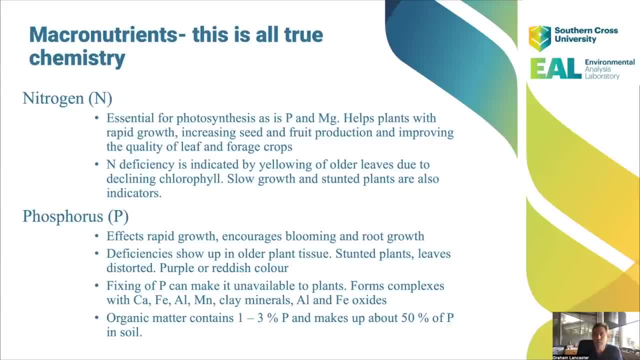 declining chlorophyll, slow growth and standard stunted plants are also indicators. so each of the elements here. phosphorus: i've got a bit more of a description there and really this is information that's very valuable but it's not essential with biological farming, if you're. 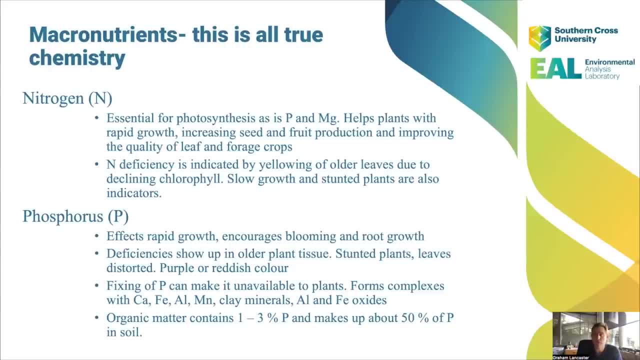 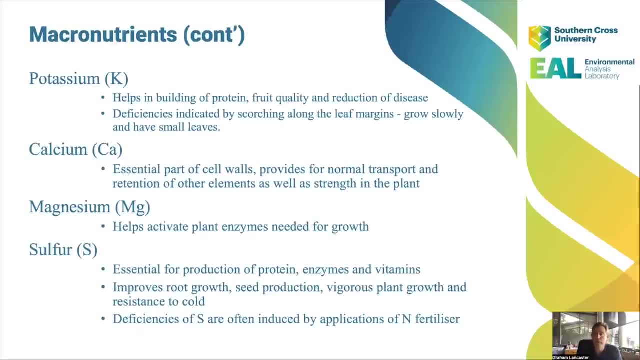 building a healthy soil, which will then create healthy plants. so this is only if you've got problems. you're starting to look into these things and we want to feed all these nutrients- and here's some more here- with a good compost supply that's got these elements in abundance. so i won't go through all these in detail so you can read them. 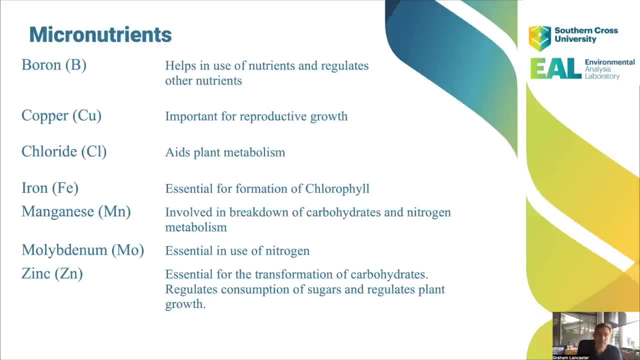 here, and even um. you have your chloride. that does aid in plant metabolism, but only in very, very low concentrations. your boron: as i said, it's very leachable element. we have a lot of soils in australia that are very deficient in copper and zinc, so all that's saying is that you need to have a balance of elements and nutrients in your soil. 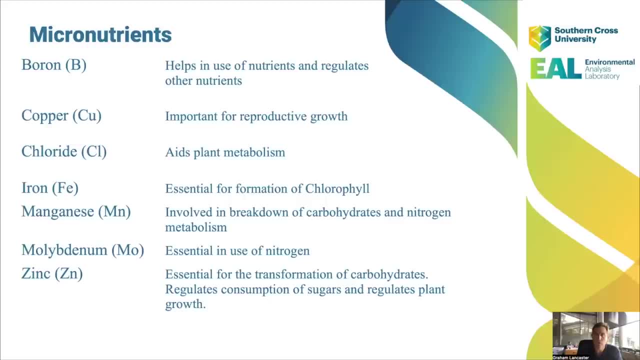 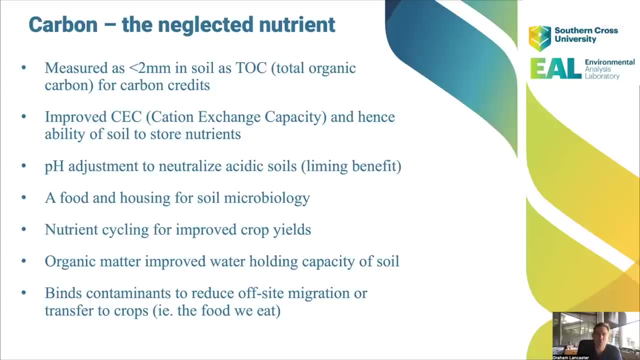 in your farming system and you can't just rely on soil biology. they can't create these elements. these elements must be supplied, whether by small additions of fertilizer or by compost- and look, i haven't really mentioned compost, but you can have additives in compost. so i like to 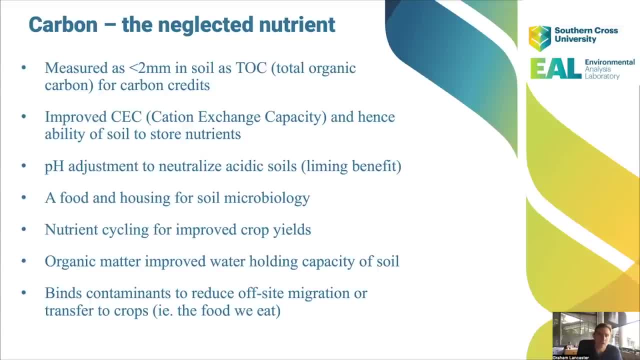 suggest you can add lime, or you can add some rock phosphate, or you can add some- i'll talk about rock sap- into a fertilizer at the start, or some biochar, just to add in elements that might be deficient in your soils. so you need to know your soils- carbon. i just talked about all these different. 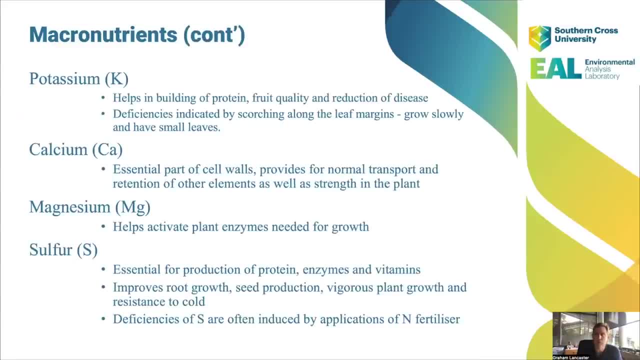 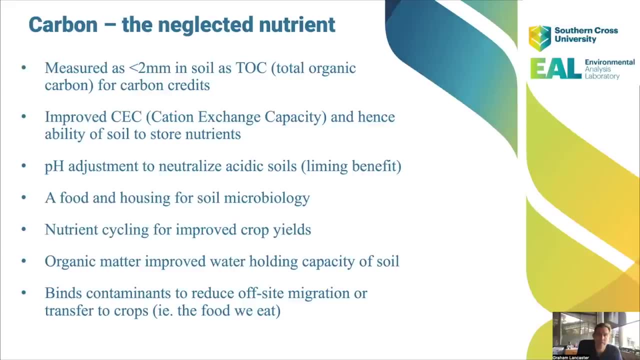 things and macro and macro nutrients. nothing in traditional farming even looks at carbon. carbon is such an important element and i believe it's been totally neglected in the past. it's measured in the lab is less than two millimeters. if you think about two millimeters, it's tiny. it's not the organic matter you can see in your soil. it's this organic matter you. 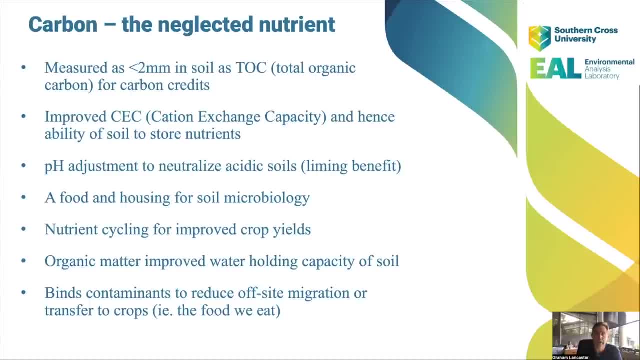 can't see in your soil that we call the carbon of soil, total organic carbon, and it's what is involved with carbon credits. improved cation exchange capacity- and it's a very chemical term i'll go through shortly- is given by increasing organic matter and organic carbon in your soil. 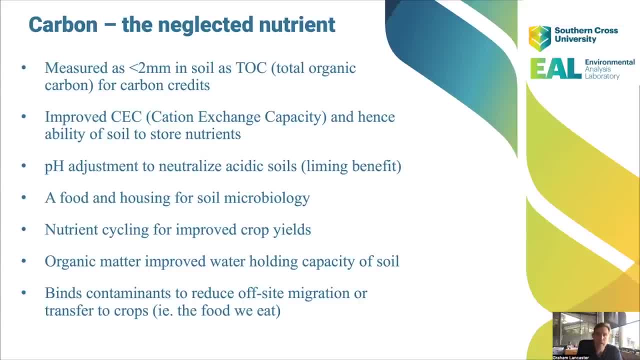 and hence the ability to store nutrients. ph adjustment to neutralize acidity is, once i just mentioned before a soil and housing for soil microbes. so if you build up your organic matter and organic carbon, it's, it's just building up your soil and allowing housing for your soil microbes. nutrient cycling for improving crop yields. um, like i was saying, 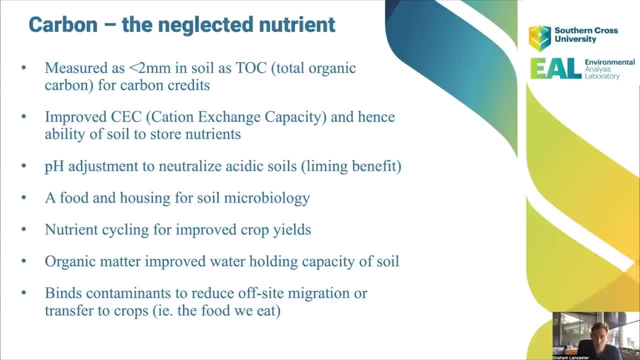 before increasing the store of nutrients. organic matter improves water holding capacity of the soil and there's lots of papers and published data on this. binds contaminants to reduce offside migration or transfer to crops. we don't want these elements- heavy metals or pesticides- in our food that we eat, even though we know it's there. we need to improve all that and that's where organic 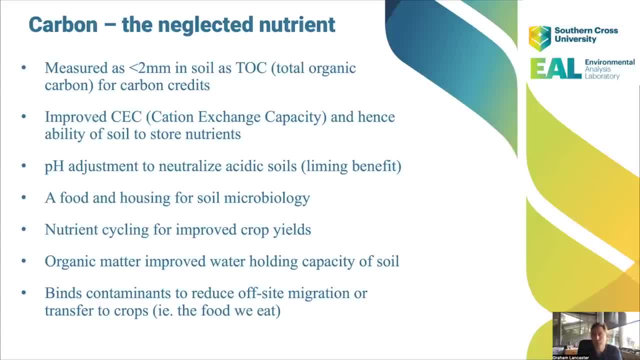 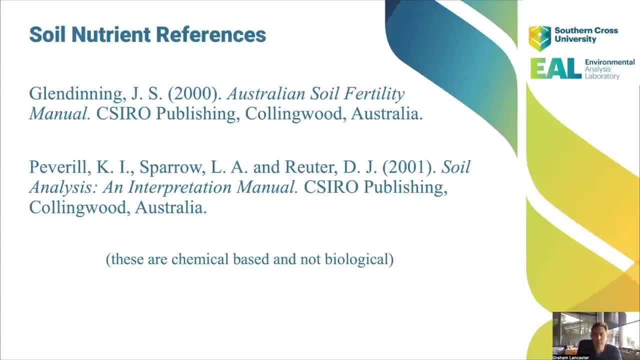 carbon can also play a big part in the conversion from industrial to biological systems. some soil references here if you want to have a look more at the chemistry side of things. um, you've got here an australian soil fertility manual. may sound good, it doesn't give you a lot of information, sorry. 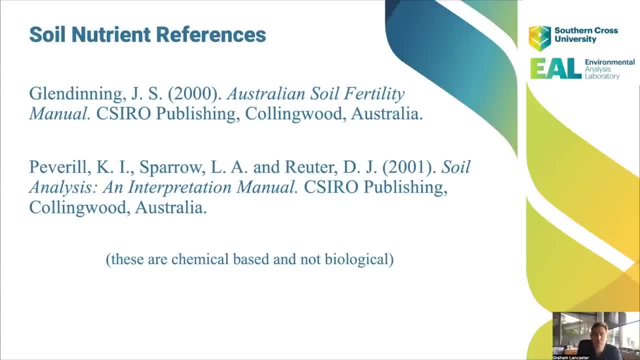 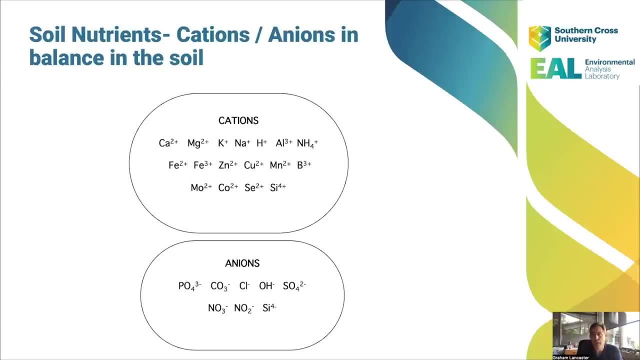 soil analysis and interpretive manual. it talks a bit about the chemistry but it does not have the answers. even a lot of your traditional farmers that read these are a bit disappointed, but they do give some information. if you feel you're a little bit lacking. they're not biological related, these publications, to really talk about soil. 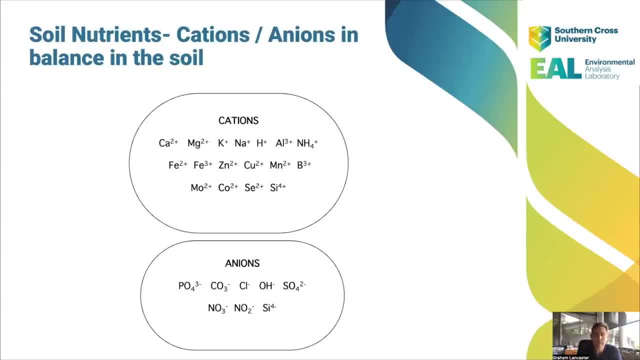 chemistry. you've got to understand what your cations are and what your anions are. they run in balance, they run in oxides, or you can see your oh there, your carbonates, that's your anions. your phosphates, they're all your anion compounds. your no3 is your nitrate. 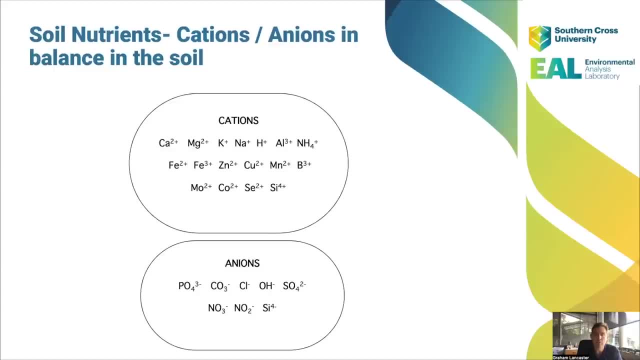 you know two's: your nitrite um, and you can see up there for your cations. your calcium, magnesium, potassium, sodium hydrogen, your acidity in your soil, your aluminium, your ammonium, ammonium, mine ion 2, iron 3, zinc, copper, manganese, boron, molybdenum, cobalt, selenium, silica, and the list goes on and on. 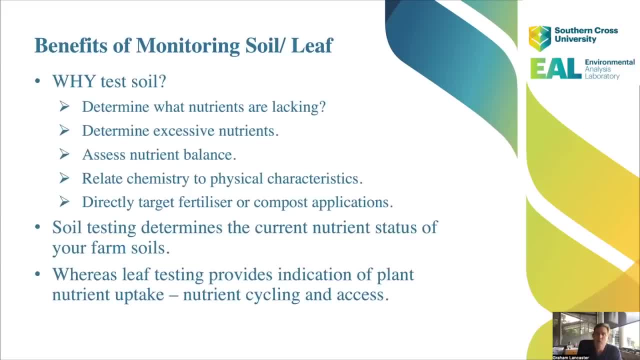 Benefits of monitoring soil and leaf or why test soil? We take a whole different concept here. We want to see what nutrients are lacking, not just to determine what to add to the soil and to sell fertilizers, because we have no association with any fertilizer companies. We just want to make 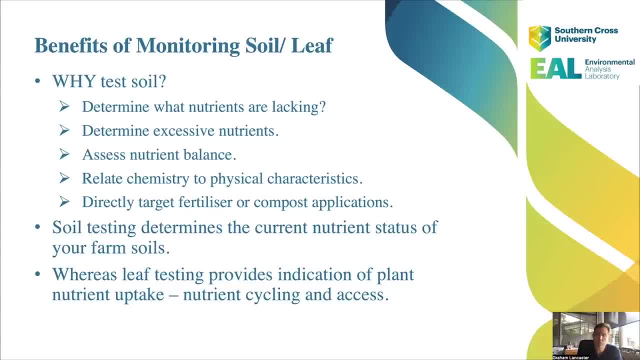 sure that you're not going to get a deficiency To determine excessive nutrients. really, if you've got excessive nutrients from historical use of phosphate, superphosphate or urea or whatever, you need to know that so you're not putting more and more on To assess your nutrient balance. 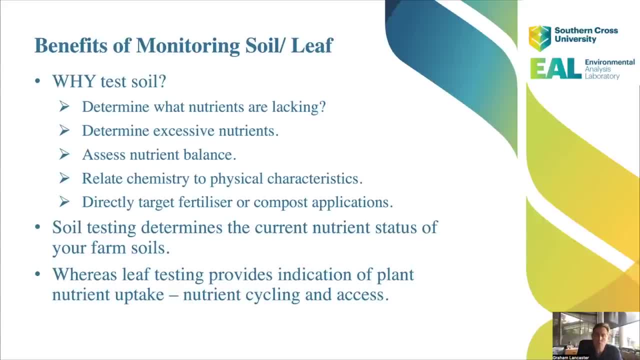 and I think that's a huge part of it I'll talk about shortly. To relate chemistry to physical characteristics, Your calcium to magnesium ratio does, I believe, impact your soil physics and your compaction in a lot of soils, and I think that's ultra important as well. 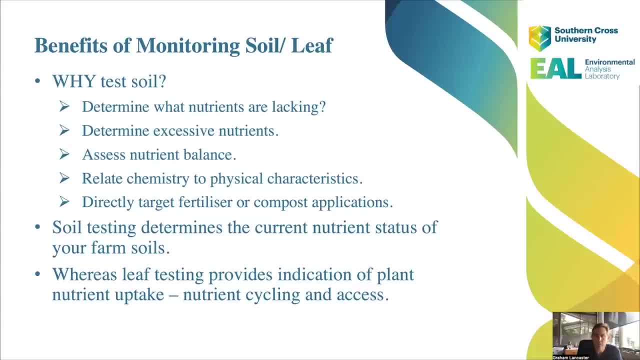 Directly target fertilizer or compost applications. and I was saying that before. If you really do know your soils are zinc and copper deficient, then adding some micronutrients, as in some zinc and copper compounds, into your fertilizer so that it binds up with the soil biology and makes a rich 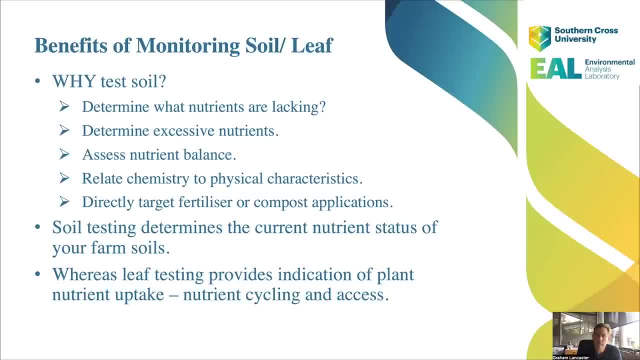 compost. Soil testing is done to determine the current nutrient status of your farm soils. Leaf testing is done to look at providing indications of plant nutrient uptake or nutrient cycling and access of nutrients. They give totally different things and when I see agronomists selling one or 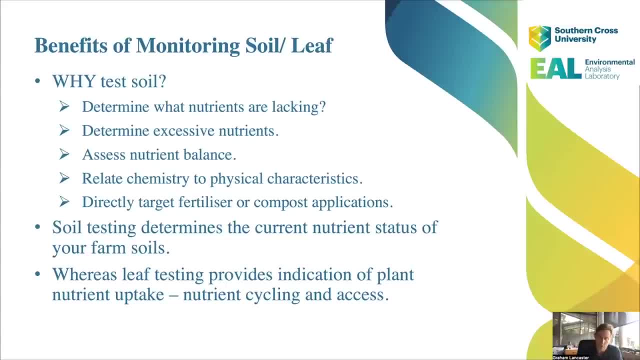 the other. I think they really just work together in conjunction And really a low cost tool in both cases to determine whether you've got issues and what you need to look at in your farm Once again if you're purely a very successful biological farmer and you've got great nutrient. 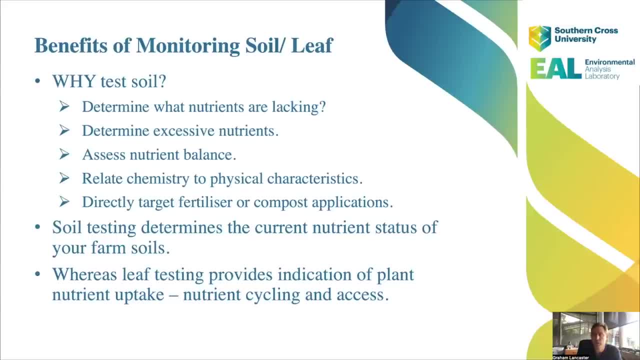 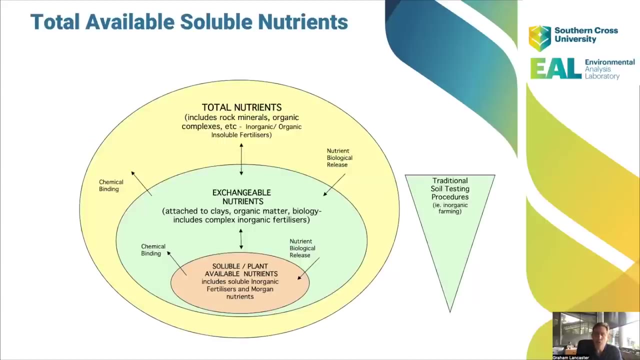 cycling happening and you're out there feeling, touching your soils, looking at your plants, looking at your crop production and your plant production and your plant growth, then really these are minor concerns and you might only test very rarely. Well, we have pushed a lot in EAL. 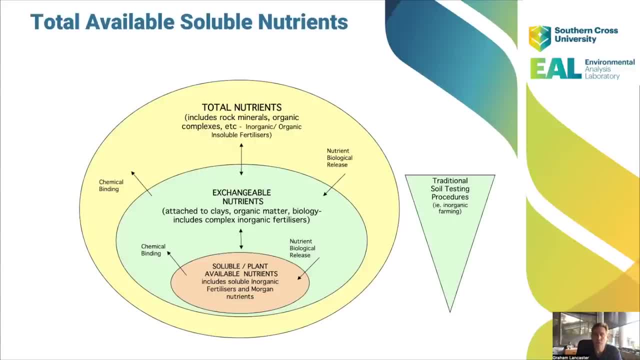 It's really the total available and soluble nutrients. So total. we look at your total acid extractable. So boiling acid with your soil to look at what stored nutrients you have. what stored phosphorus, potassium, calcium, magnesium, right through a big list of micronutrients as well, Even things. 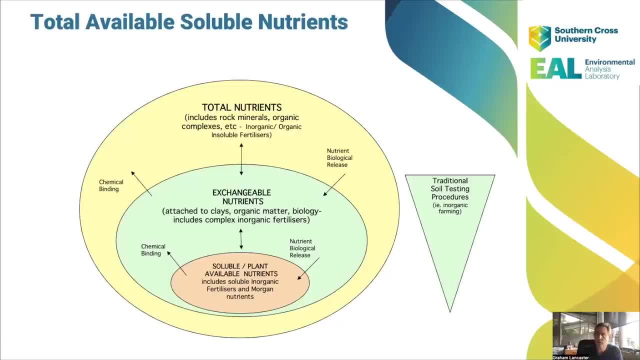 like your zinc and copper, which I've mentioned a couple of times. There's a big store of those, but not in all soils, So this is also related to your soil type And I talked about your soil texture. Generally, the clayier your soil, or the higher organic matter in your soil, the bigger this. 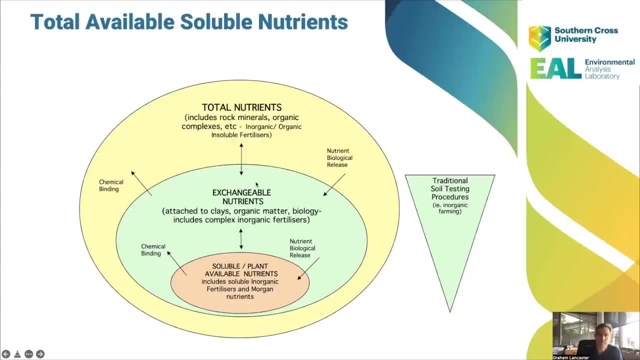 pool of nutrients is in your soils And then you've got your exchangeable nutrients, and that's which is traditionally looked at in soil testing labs. They don't even look at these totals. They don't want to know about it, but there's a big cycling that occurs between exchangeable and total. 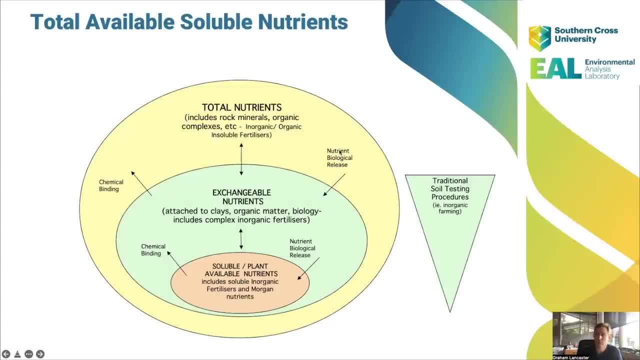 and total to exchangeable, which is what we want to do, is to get this nutrient biological release. There's always going to be chemical binding, but we want to reverse it with bringing the soil biology into the process, And then you have your soluble nutrients. So you've got the soil you've. 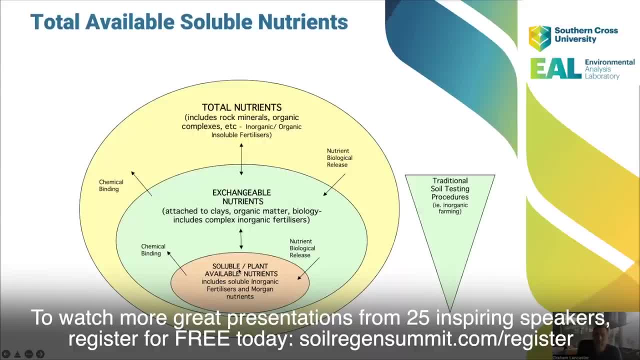 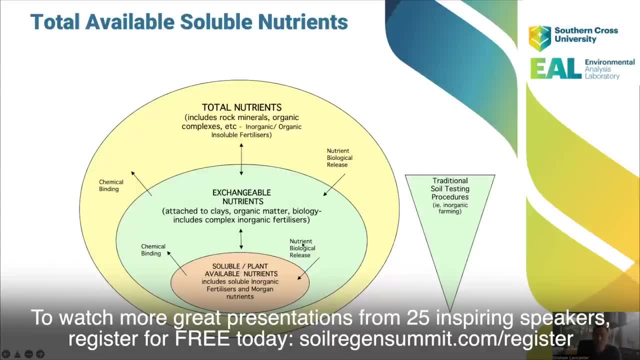 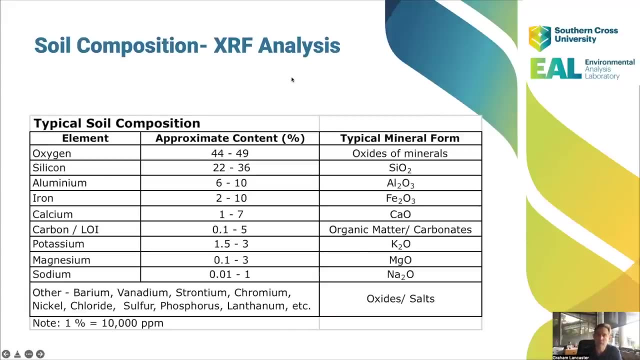 through, solubilize some of these nutrients with the soil biology and release it to the roots through biological processes, which is what we're relying on. I talk to people about the actual soil composition and I think this is important to understand. X-ray fluorescence analysis, or XRF. 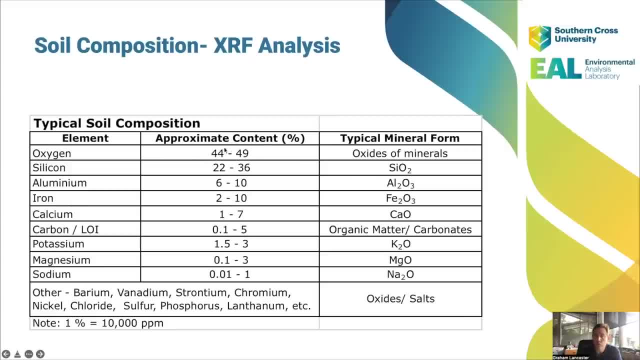 if we do a typical soil, oxygen is your major component of it, of your soils, and that's your oxides and minerals. So this is your silicon oxide, aluminium oxide, iron oxide. Your next most abundant element is silicon. It doesn't mean you've got loads of available silica or silicon. 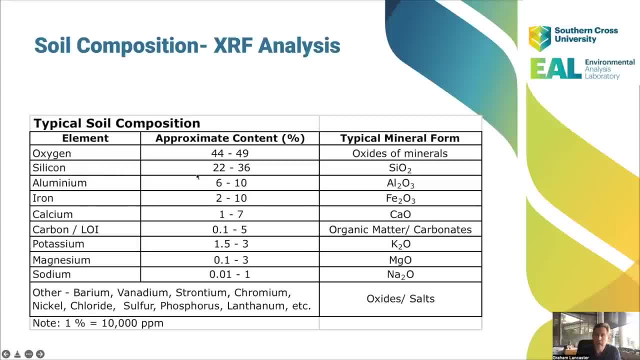 but it means it's mostly bound up as silicon, as silicon oxide, which is your clay, your silt and your sand, The whole structure of your soil. The aluminium is hugely abundant When I say 6% to 10% aluminium. 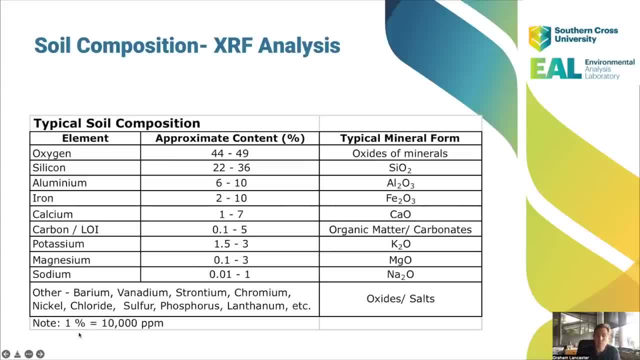 in Australian soils, or 2% to 10%. we're talking. 1% is 10,000 parts per million or milligrams per kilogram. Parts per million and one milligram per kilogram are the exact same unit, So you've got to. 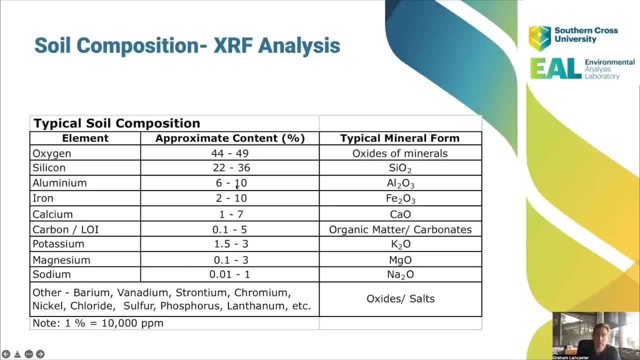 understand units to some extent And a 6% aluminium in soil is 60,000 parts per million Or 60,000 milligrams per kilogram With. looking at calcium, it's very variable Carbon. a lot of Australian soils, especially inland New South Wales and Queensland and even Victoria can be. 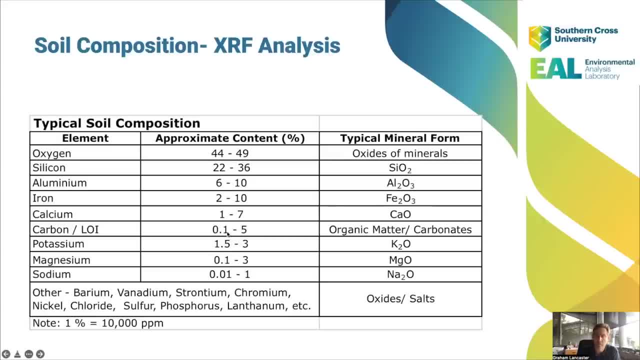 down to 0.1 or 0.5% Carbon, organic carbon, which is extremely low levels. We want to see organic carbon well above 1%, Nice to be up to about the 5% or even higher. There's no limit. 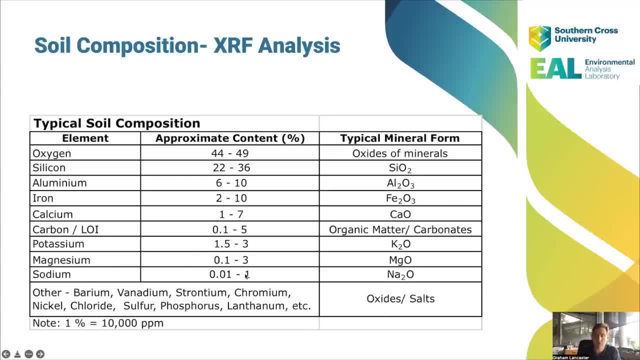 Potassium, magnesium sodium. you don't want that too high, as it gets toxic. But then there's a whole range of other elements- barium, vanadium, strontium, chlorine, nickel et cetera- that are 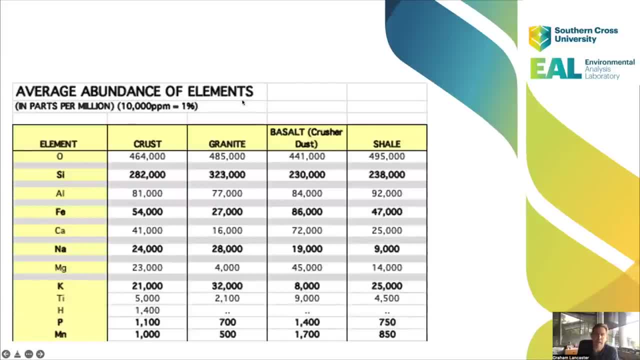 present in soils. It's interesting that the average abundance of elements in the earth's crust in granite, which is a mineral, basalt, which is crust of dust in Australia, and shale- these are three typical bedrock type materials- You can see the average abundant elements there And that's the raw material It's leached out over. 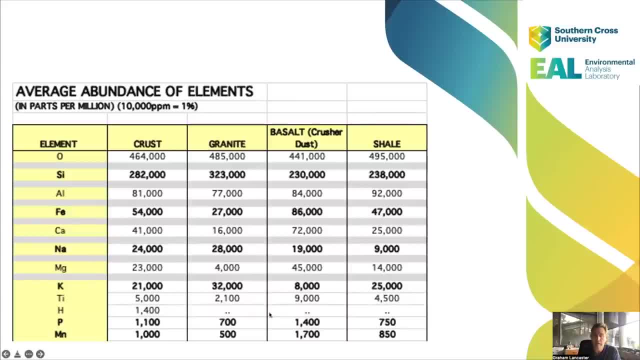 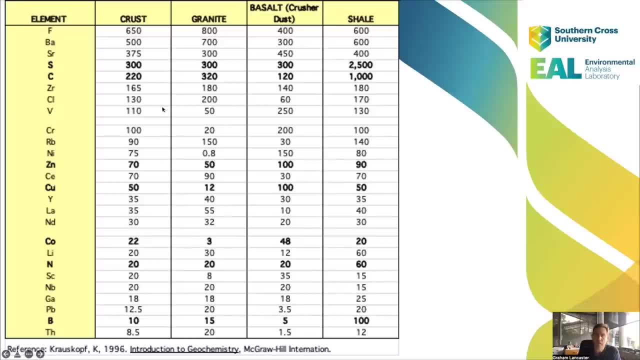 the time, over millions of years. But that's the sort of minerals you're dealing with. But the thing I want to note here is: look at all these elements. we don't even think about Caesium, yttrium, lanthium, rare earth elements, even toxic elements like arsenic, chromium, nickel. 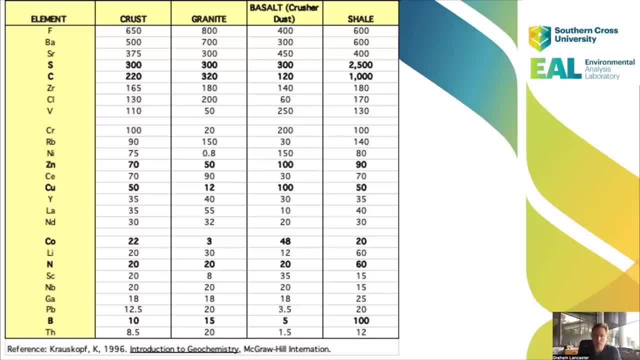 they're all naturally occurring in the earth's crust. They're all naturally occurring in the system, the system. So what stage do we see? Well, actually, this whole process, biology and process, a plant needs tiny amounts of these elements. I know some radioactive elements like uranium, strontium just, also quite abundant in Australian. 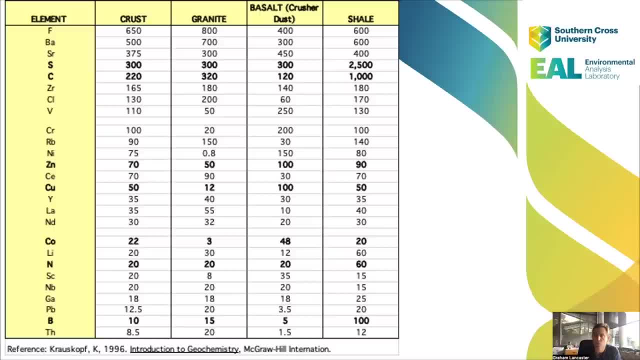 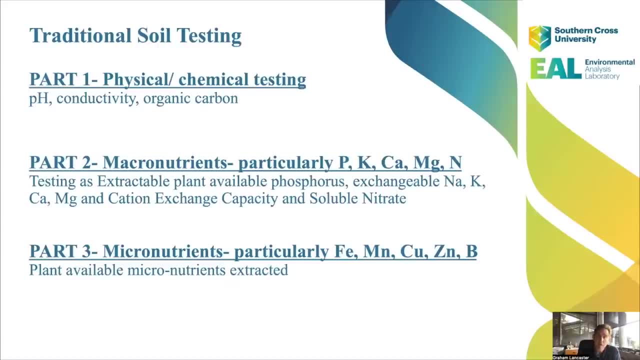 soils, and maybe that's good for ancient soils, but I'm sure they're also present in soils all around the world, So it's a bigger part of the picture. So, traditional soil testing, الل, it really just has your part, one which is your simply, your ph, your conductivity, or your ergs, or 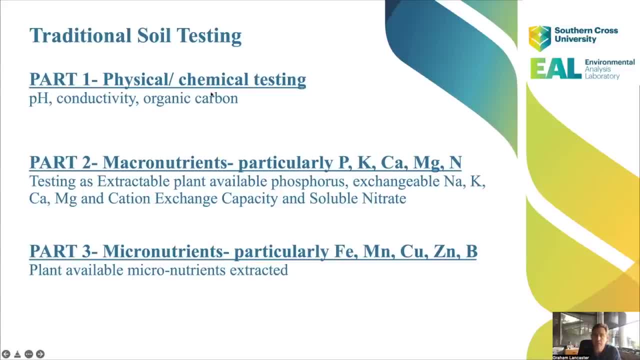 your salinity of your soil, your organic carbon, and i think that's so important to test. then part two is your micronutrients, particularly phosphorus, potassium, calcium, magnesium, nitrogen, and they're normally just your soluble nitrate. they don't even look at soluble ammonium. 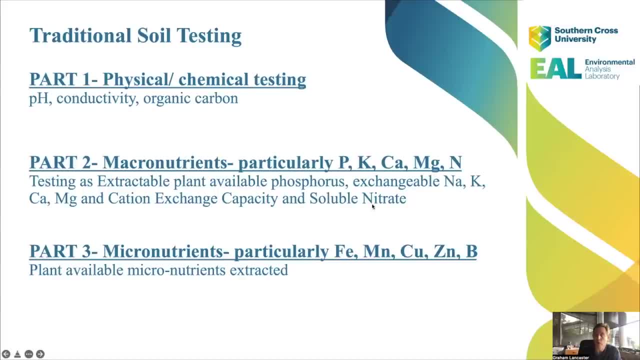 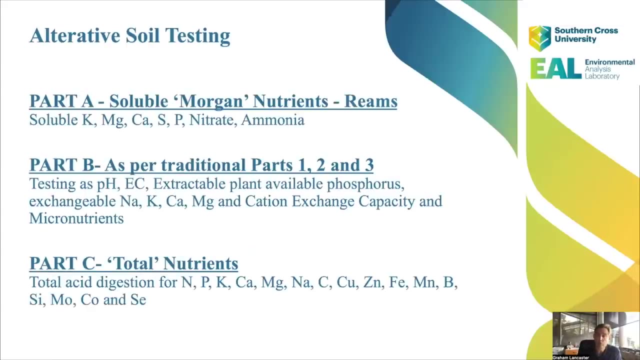 and they don't look at your total organic nitrogen, which is another aspect i'll talk about shortly, and then your micronutrients, which is primarily your iron, manganese, copper, zinc and boron. alternative soil testing, what i've already mentioned, is really what we do primarily in. 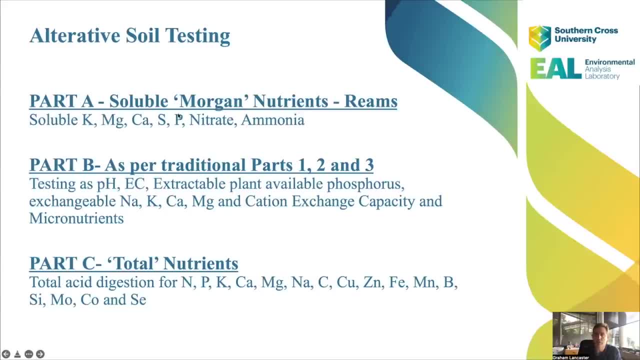 eal, which is looking at, is soluble and morgan extract is a reams extract developed in america. we've adopted here, just to look at these soluble nutrients, your soluble- potassium, magnesium, calcium, sulfur, phosphorus nitrate, ammonia, then your traditional, which is really just back to that previous slide, part one, two, three, um looking. 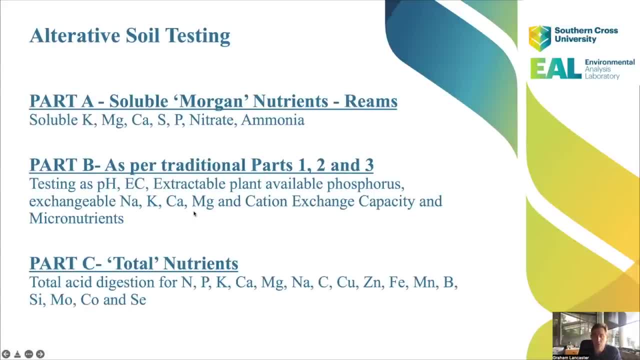 at ph, i won't go through that again. exchangeable cations, micronutrients and then the big part which we like to know is your total nutrients and, like i said, the reason we want to know that is we want want to know we've got a safety net in biological farming that we can rely on these total. 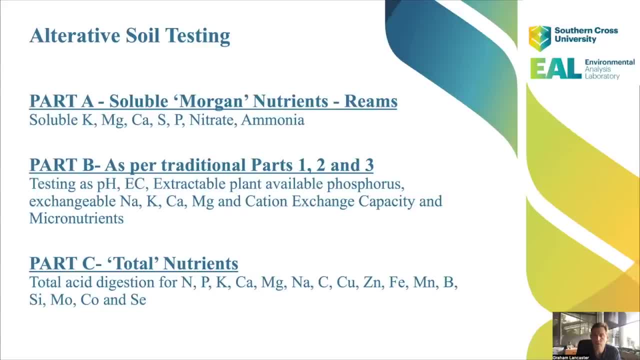 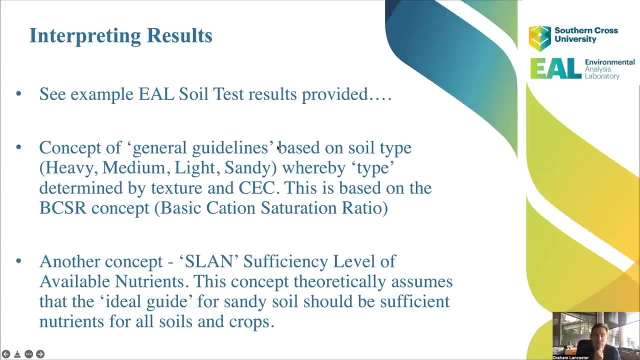 nutrients to access them with our biology. so we're taking off our total dependence on synthetic fertilizers, and that's what really i like to push. interpreting results: that's a whole nother presentation, um, and look, it's not simple, it's chemistry. um, i love it, um, but it does take a little bit to get your head about, so i'm happy. 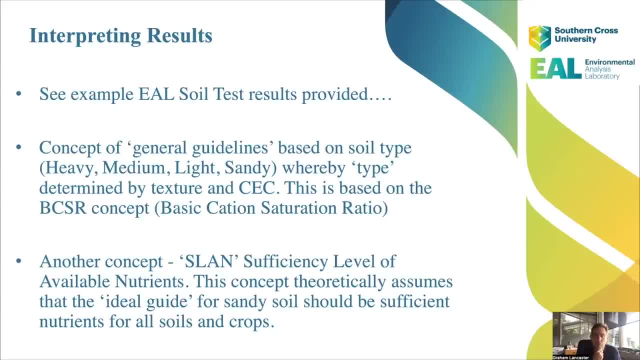 to answer questions there and i'll go through it briefly now, but i i'll go through a bit at the end where i've got an example eil soil test here, and then at the end i'll talk about an example interpretation sheet that i'm sure can be provided. i go on two concepts. one is a concept of general guidelines based on soil type. 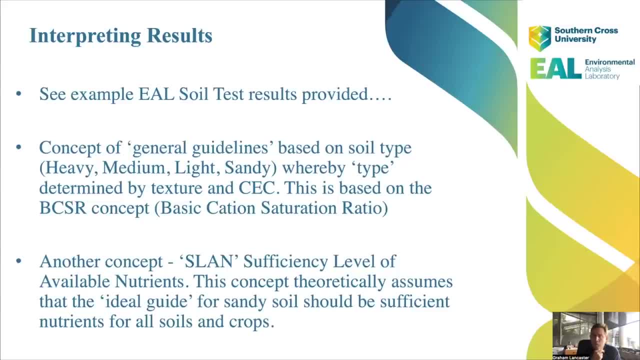 and i think this is important. a lot of agronomists go on what you're growing, but i think it's irrelevant to what your soil can hold if you've got a heavy soil type, a medium soil type, landy, light soil type or sandy, and this type determines how much soil you're going to want to grow, and so 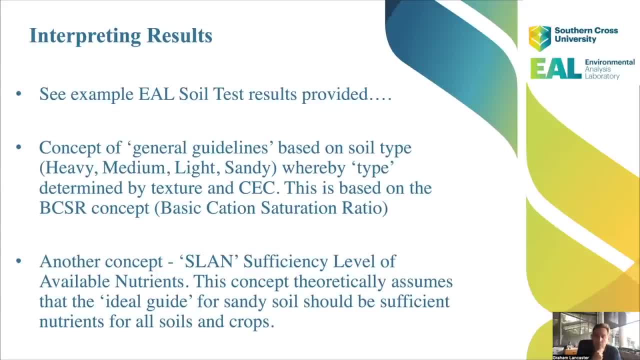 it's important to understand that the soil type is determined by your texture and your cation exchange capacity, which i'll go through shortly. so your clay soil, your heavy soil, is a clay, or even a clay. heavy clay loam will often have a cation exchange capacity above 20 milli equivalents. 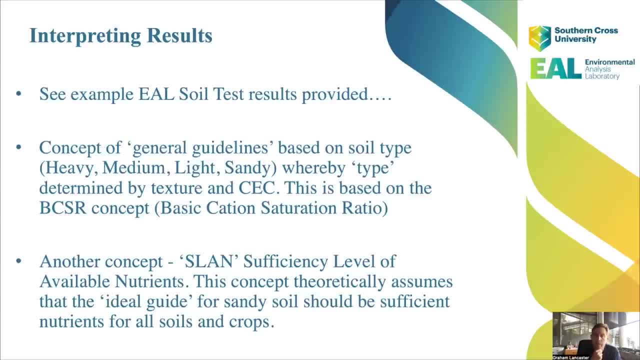 per 100 gram or micro siemens per centimeter. there's different units there, but generally above 20.. and we had some soils in australia- heavy black soils- that maybe have a hundred cation exchange capacity- 100 milli equivalents per 100 gram and this is based on a basic cation. 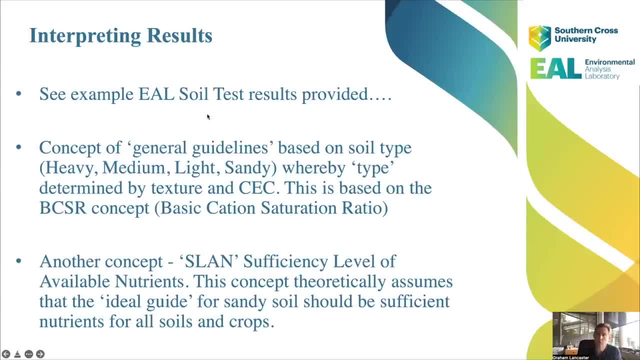 saturation ratio and this is balance: balancing out your cation exchange ratios and basing that on soil type. another concept i think is very important for biological farming- it's called slam, or that's a name for it- sufficiency level of available nutrients and this concept theory. 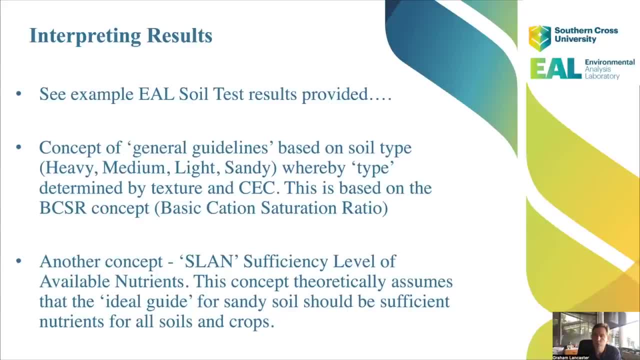 radically assumes that the ideal guide for sanding soil should be sufficient for nutrient for all soils and crops. so basically, i'll show some guidelines in a moment. a sandy soil holds less nutrients, has less expectation of nutrients, but crops grow in sandy soils. so really, a concept there is. 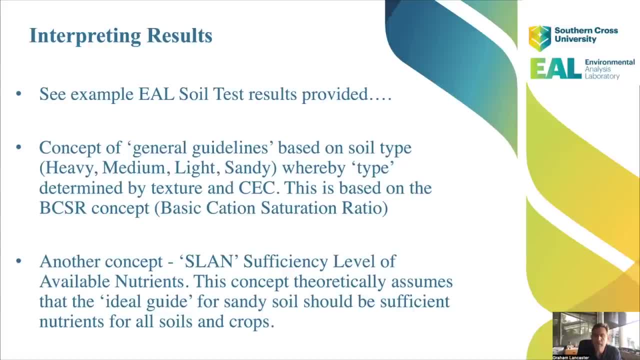 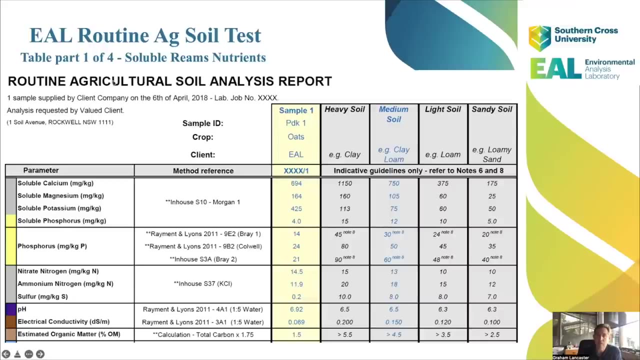 the amount of nutrients. if you've got that in any soil type in there, it's enough to grow a crop. but really you you want to try to build it to a level that that soil can sustain and hold on to it in your soil profile. so i've just got um a few slides here, um on, and this is part one of four. 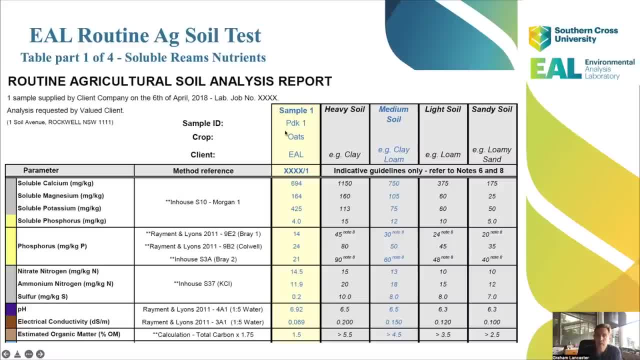 because this is one soil test in eal um where we have an example which is an oats um in yellow here, and four soil types: heavy, medium light and sandy. so here i've made medium blue and i'll flick through some slides to explain why i've selected this guy. 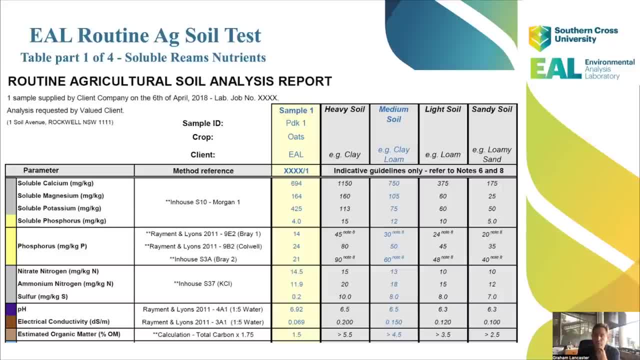 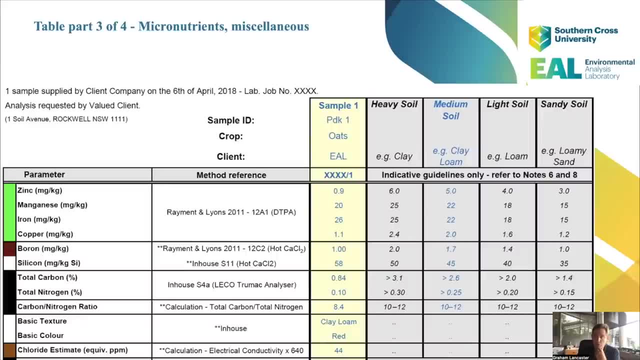 line, so you don't look at the other guide lines, because i'm saying this soil type and i'll go through the reasons why. um, basically, if i go through two slides, when we've textured it by hand, it comes as a a clayloam and that's a clay loam. so 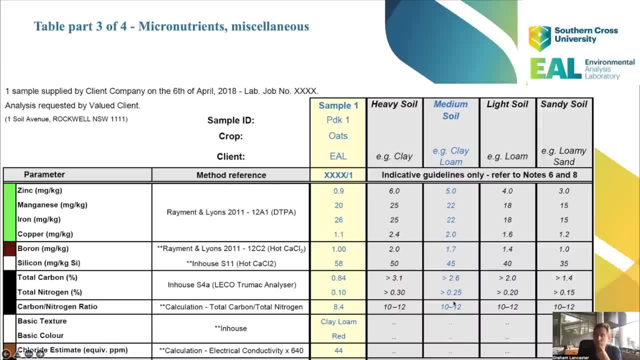 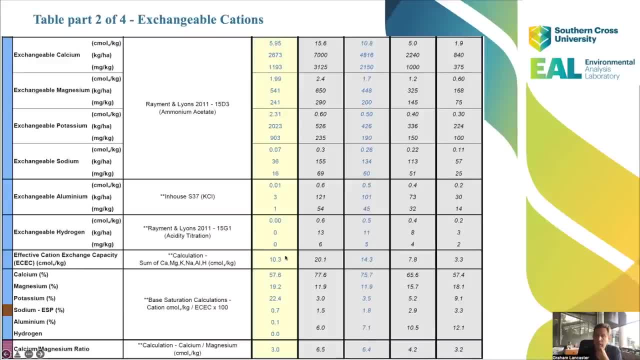 medium soil type. so we're saying that's where it should be. that's the first indicator of that's why i've picked these guidelines. the second is: when we measure that soil, it comes to a 10.3 cation exchange capacity or effective cation exchange capacity, which is the 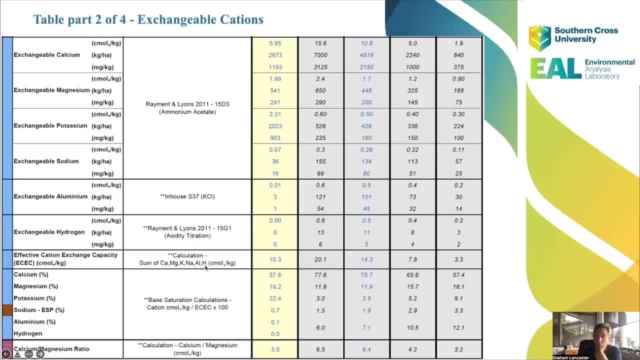 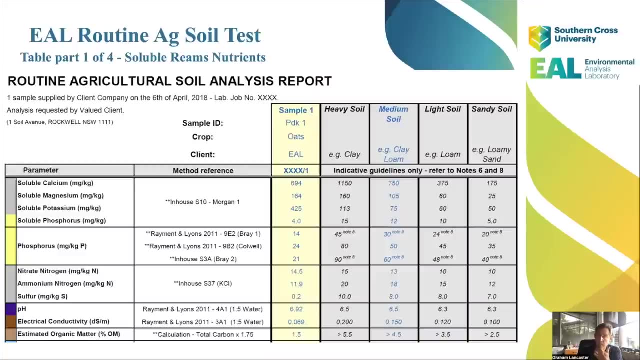 sum of your calcium, magnesium, potassium, sodium, aluminium and hydrogen, and i'll go through that in more details. this is complexity of soil testing. it comes to 10.3 now- that's between your 14- as a guideline for your um medium soil and 7.8 for your light soil. but we've already 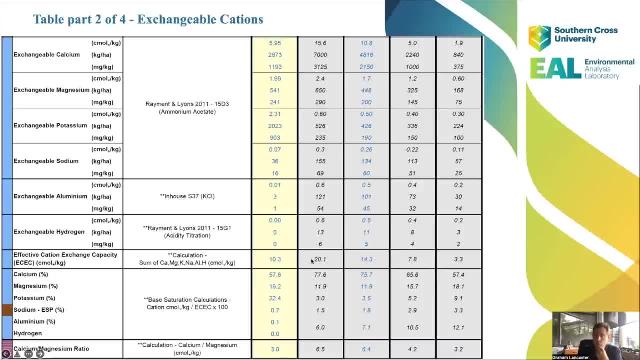 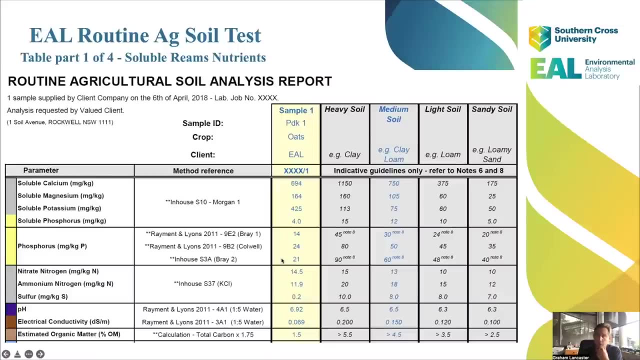 said, the texture is more towards a medium soil and really even instantly. that's shown that soil is deficient to what it's capable of holding, of what its cation exchange capacity is capable. it's not reading as high as it should, so i'll go back to that previous slide. this is part one. we've 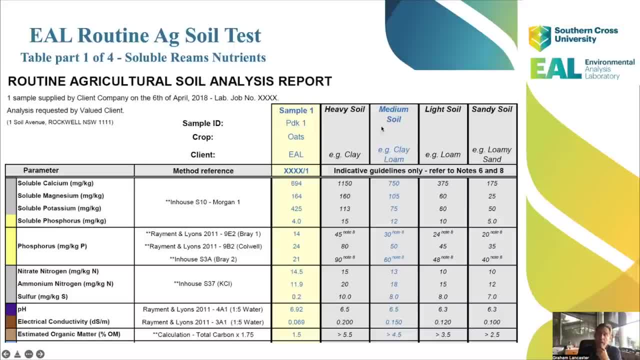 selected this medium soil classification um, and then we have our oats. so now it's simply just looking through what's your soluble calcium, magnesium, potassium- you can see that's way above the guidelines. you never need to add potassium to this soil for i won't say forever, but for years. soluble phosphorus. 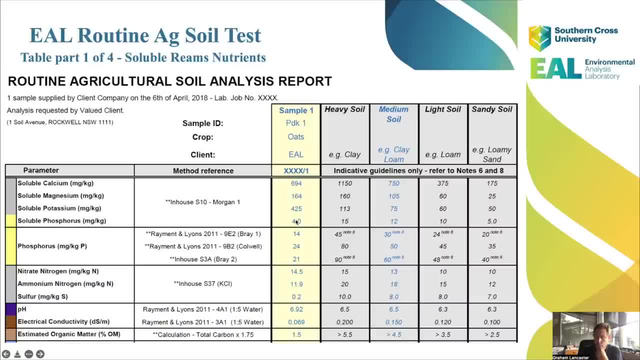 is very low in australian soils. we just can't get our soluble phosphorus very high. we have so much iron and aluminium in our ancient soils it just binds it very quickly. so we actually do need either super phosphate, which we don't encourage, or a good soil biology to get that. 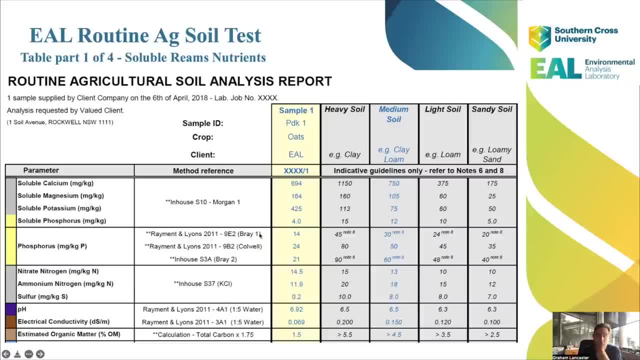 type of soil. so we use a little bit of liquid toxin so that we can get a very good soil選 toöde in the soil. so i'll give you the example. i'll show you what that looks like. um, as a general idea. so as an example, here's our work. so you get on here. we have a one day. 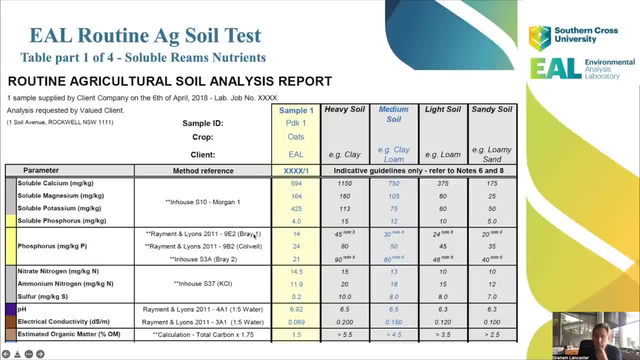 a one hour basis. you can get that the first three months. so in fact your per year one and two weeks. you get to a level each year where the soil will be a little bit more sustainably. so you can get that a little bit more than the first year. you can get a little bit more storage. 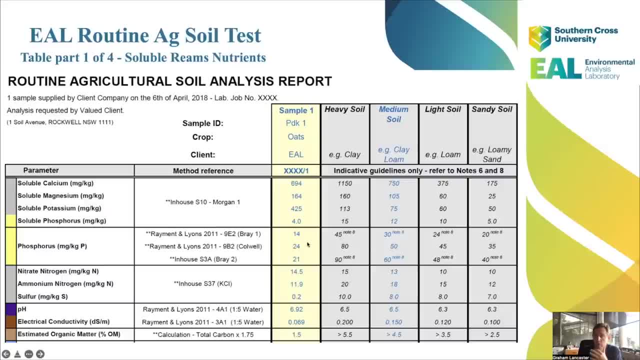 of water juice out of your plant, you can get a little bit more sediment out of your soil. so that's a higher guidelines. but you see these soils, they're close to the sandy soil, so not really that deficient. but um yeah, compared to guidelines they're showing to be a bit low and i'll go. 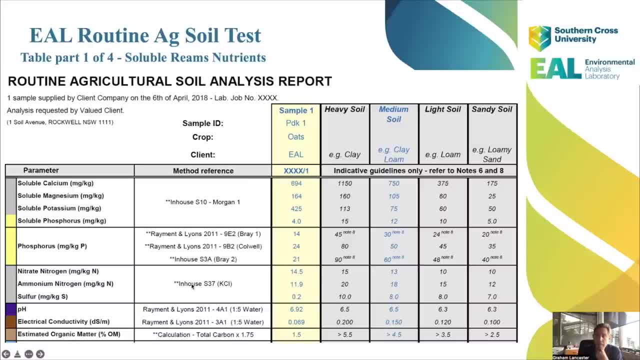 through total phosphorus in a moment. um. so, nitrate, ammonia and, like i said, i think it's important to look at them, nitrate and ammonia, because they're interchangeable- um, your ammonia can chemically convert to nitrate and your nitrate can chemically convert or biologically convert to the ammonium. 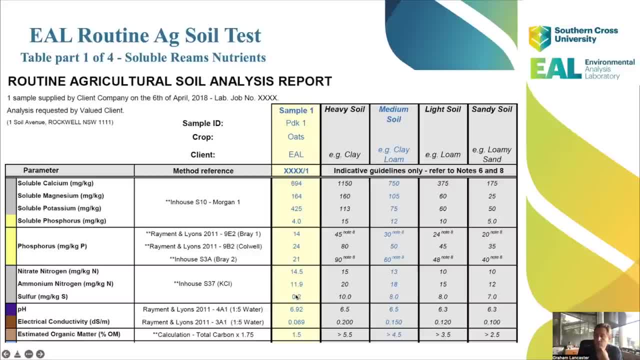 sulfur very, very low for this soil type, but, like i said, it's leachable. this soil would have been taken naught to 10 centimeters or naught to 15 centimeters, so your sulfur could be fine for your plants because your roots go lower and your sulfate's likely to leach lower as well. so 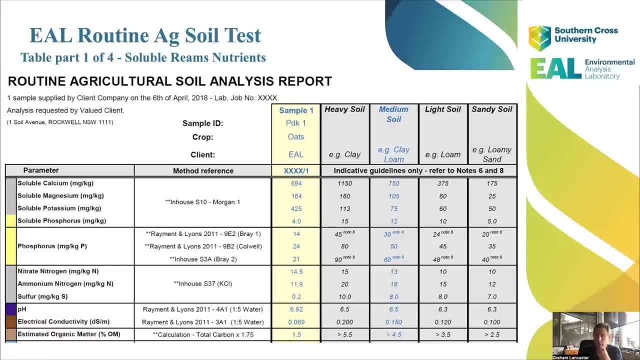 understand your reasoning, where you've taken your soil and the whole dynamics of what you're dealing with. ph is trying to be nearly neutral. 70 percent of your soil is going to be neutral, so you're going to be in control. and your nitrogen is going to be neutral, so you've got your nitrate of 0.67. 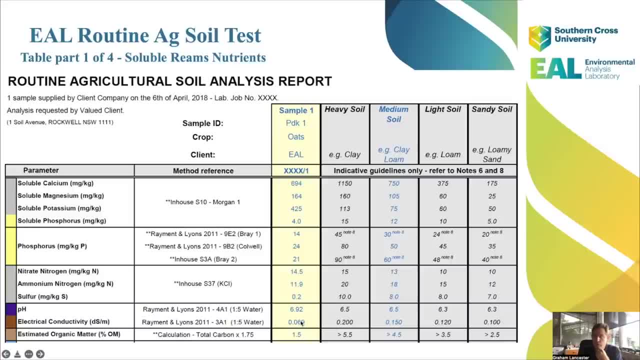 is neutral um, and then your salts: 0.069- a little bit low, but i wouldn't be encouraging putting salt on. it's got some ergs there, which is another name for it, um, but yeah, it's showing to be a little low um, which is good. you don't want to have high sodium and chloride, which is your most dominant salt. 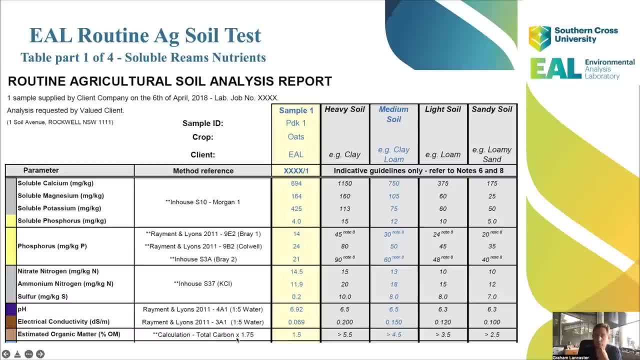 now your organic matter, um, which is actually a calculation of your your organic carbon, or your your organic carbon times 1.75, um. to cut costs, we just do total carbon in this test um, because there's typically not a lot of inorganic carbon in most soils, and we multiply it by 1.75 and you. 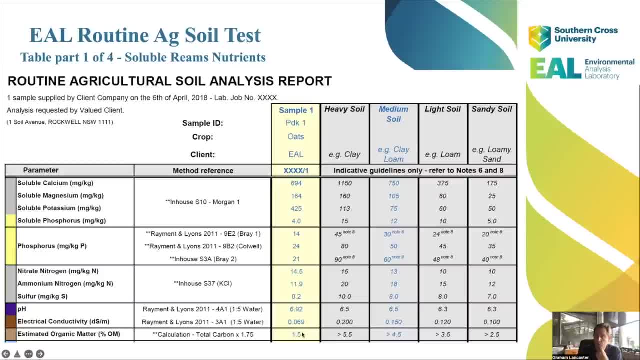 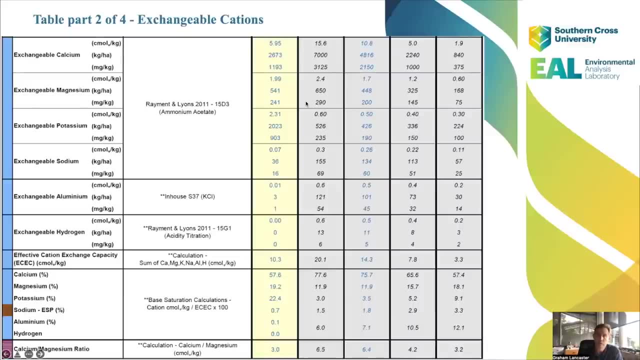 see here this soil: 1.5 percent organic matter, which is extremely low. you want it greater than five percent at least. i've had farmers say: well, what's the limit? there is no limit. i've seen soils at 10 to 15 to 20 percent, um. so yeah, you can keep going up part two of this, what i'm talking about. 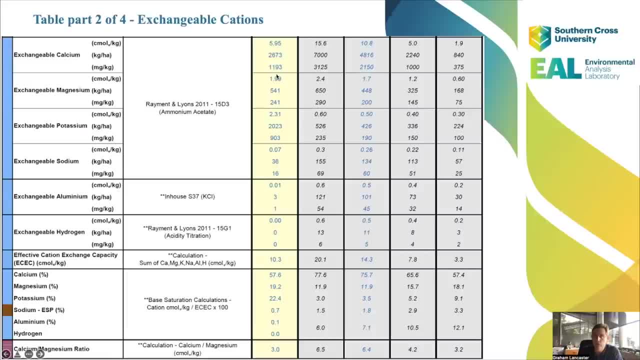 i saw test is looking at once again your, your oats and your guidelines, and just looking at your three different units for exchangeable calcium. so these are your exchangeable calcium, oh so your exchangeable cations, and you've got three different units and these convert between. 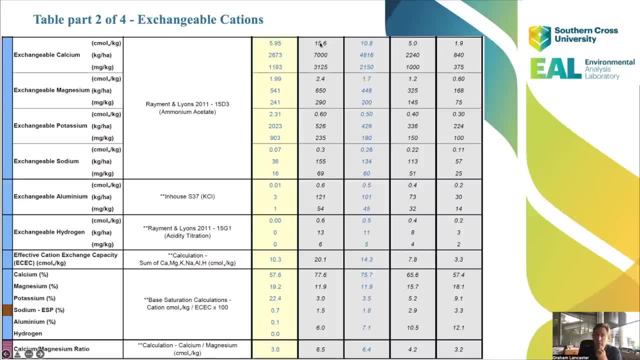 them. so they're actually the same number, just as a different unit. so here for five point nine five centimoles per kilogram is equal to 2673 kilograms per hectare, or 1193 milligrams per kilogram. it's the same value, but just different conversion. so we give all three. 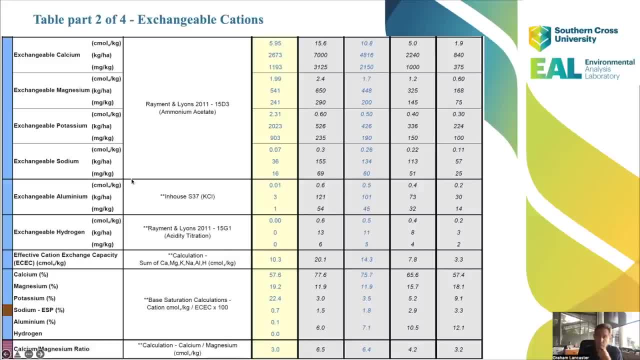 there and that goes right through your magnesium, potassium, sodium, aluminium hydrogen. and when you add all those up as your centimole per kilogram- 5.95 plus 1.99 plus 2.31, plus point 7 plus 0.01- you get your effective cation exchange capacity. and that's just as simple as it is adding. 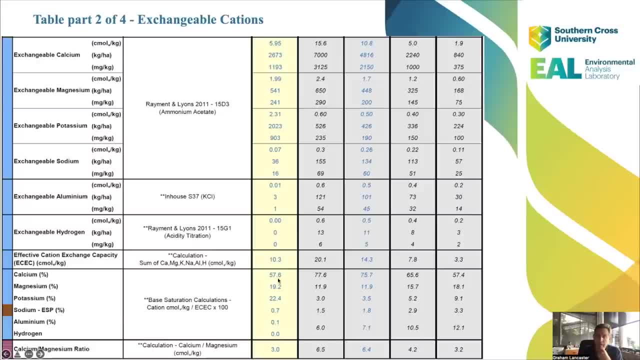 those up as the correct unit. and then when you take 5.95 divided by your effective cation exchange capacity, 10.3, that divided by- sorry, that number there, divided by that number there times 100, gives 57.6 percent. and you do that for each element: 1.99 magnesium divided by 10.3 times 100. 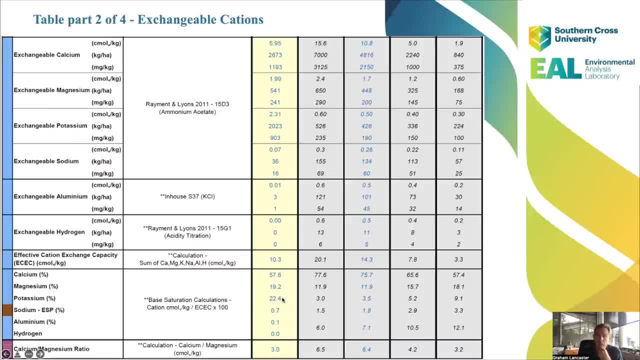 gives 19 and you go right through and then you get your balance of your cations in your soil and then you have a guidelines to say: well, obviously, looking at that, your potassium is way high. we already noted that your magnesium is a little bit high. um, but you can see there your calcium's way. 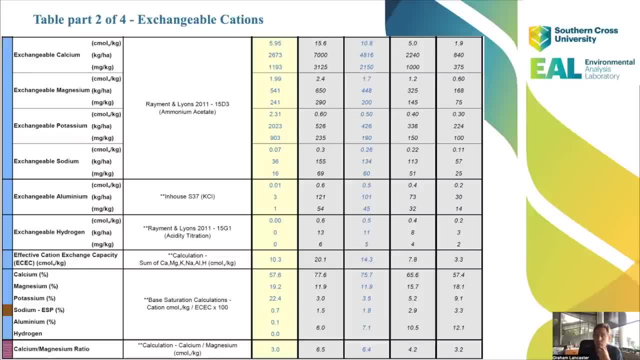 low um. so there's some deficiency in calcium and there's some deficiency in potassium and there's some deficiency in calcium there. so i often say to people: well, don't worry too much about your ph. like i said above's: fine five is fine. it's really you want to build up um your calcium, if you're. 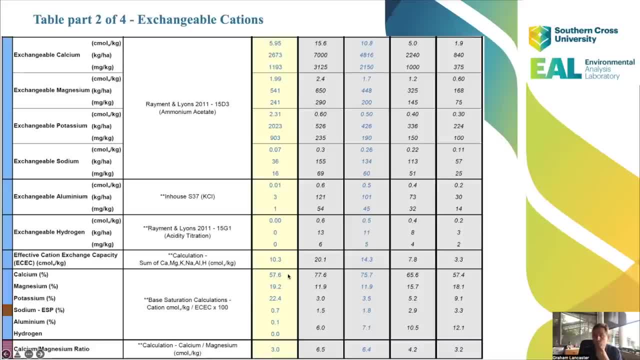 indicated. beta deficient doesn't mean you don't have a great total store of calcium, but you may also, um in this case, have a deficiency of an exchangeable calcium. and then your calcium magnesium ratio, i said in impact soil structure, indicating there to be low, which is a low calcium. 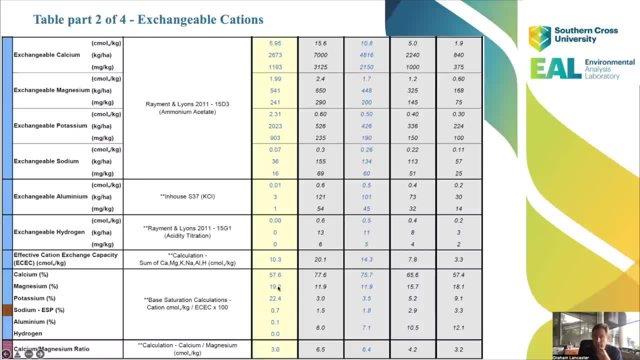 and a high magnesium. um, and you see there, the magnesium is a bit high and your calcium is very low. so, going on that- and once again this ratio is in the units of centimoles per kilogram- so you must ratio the calcium magnesium ratio: calcium 5.95 divided by 1.99, which is approximately 3 or 3. 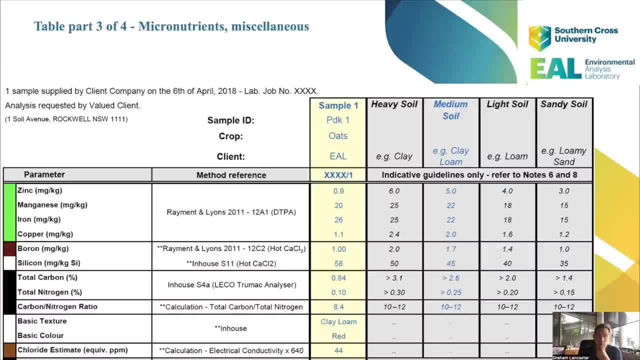 by calculation. then we go through further. um, once again, these are. just look at your micronutrients. we pick a hot calcium chloride extract for silicon to look at your available silica. i mentioned in soil, your, your silicon be tens of percent or tens of thousands of milligrams per kilogram or past million of silicon, but your 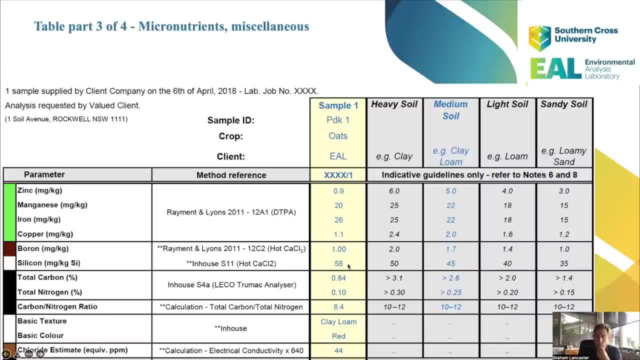 soluble silica is just another element we're finding quite important to understand the structure of the plant and the structure of your crops. total carbon here: 0.84 percent and, like as with organic matter, which i've mentioned, is a calculation- um, it's, it's very low. 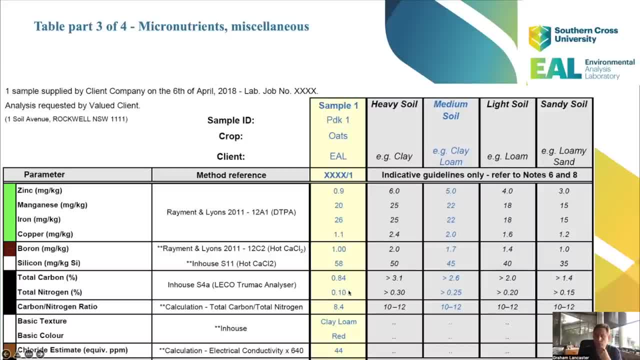 your total nitrogen is a whole nother story. your total nitrogen, primarily your organic nitrogen at 0.1 in your soil. that's actually converts to 1000 milligrams per kilogram of organic nitrogen. it's a small amount of nitro. pneumonia is included in there, but primarily it is organic. 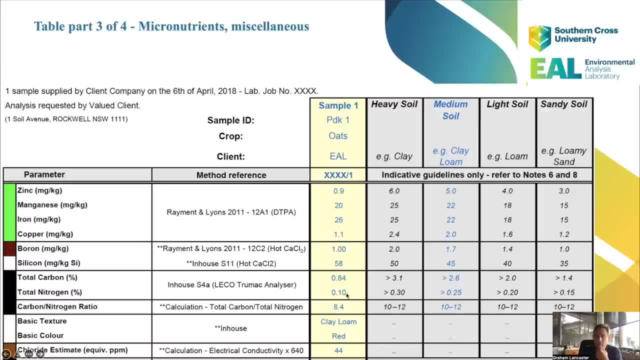 nitrogen and that's 1000 milligrams per kilogram and it generally it has a ratio of 10 to 12 to your carbon. so the soils are amazing that they they adjust themselves to this sort of ratio. in a healthy soil where they have 10 times the amount of carbon. 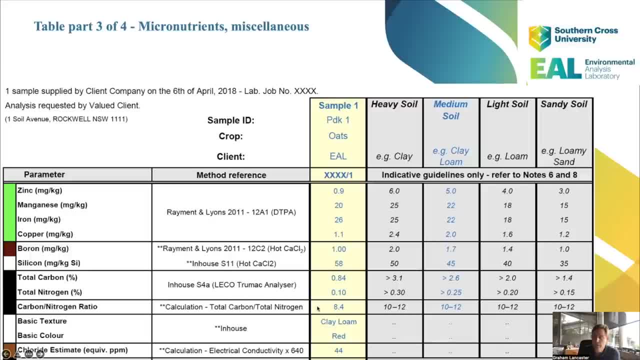 to nitrogen 10 or 12 times the amount of carbon to nitrogen, and a lot of that nitrogen, i say, is organic nitrogen and a lot of that carbon is typically organic carbon. then we just have a description here. Chloride: it's mainly looking at the toxicity of chloride in your soil because 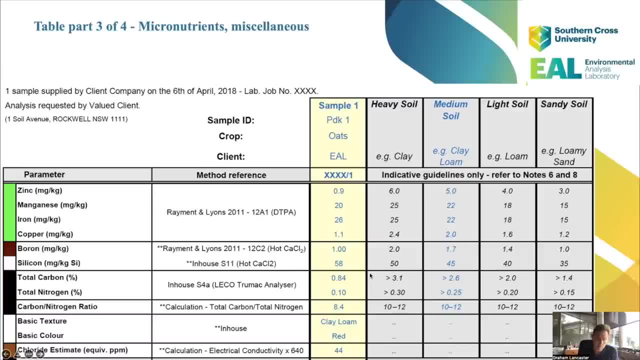 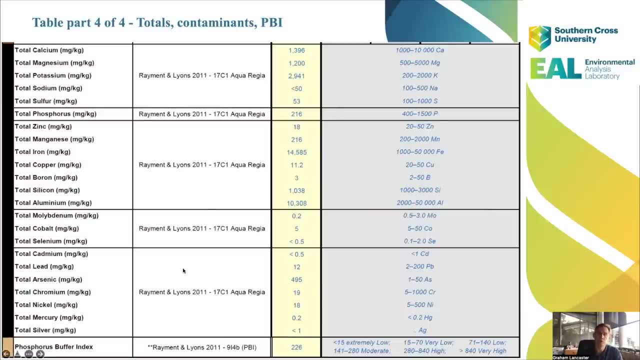 that can be a real problem with toxicity of sodium, And it's one of those chemical aspects you need to understand because it can be a major restriction to biological farming. if you do have this toxicity of salts, Then, just to finish up part of this, your total nutrients, And this is where I'm saying 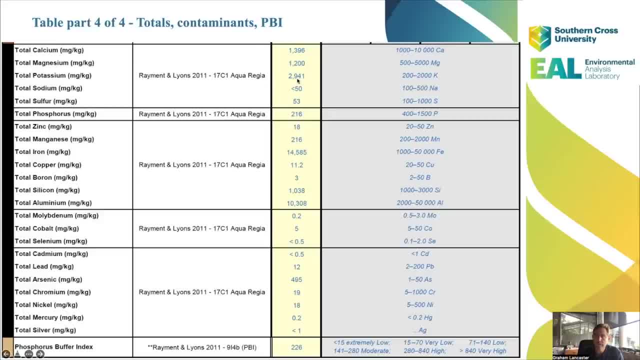 about the store. Total potassium here: 2,941, a general guide here for all soil types. These lower levels are really for your sandy soils. These upper levels are really for your heavy clay soils. So you can see there calcium's quite low magnesium. there's a fair amount. 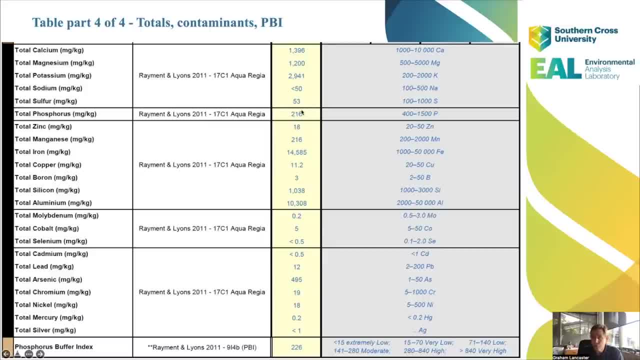 of store, potassium. it's loaded. Your total phosphorus here- 216, I would say, is very low. So I mentioned before that your exchangeable phosphorus is low. here. your total store of phosphorus is extremely low. so you've got to look at getting something in there- rock, phosphate, a mineral, whatever you can to build. 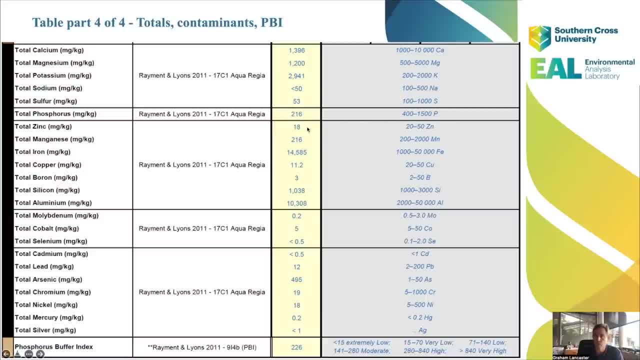 up that store of total phosphorus and that's where it's useful. zinc: you might have one or two parts per million of available zinc in your soil, but your total zinc, as here, 18, your manganese, your iron, like i said, is very rich in soils and aluminium is very rich in this soil- 10 308. 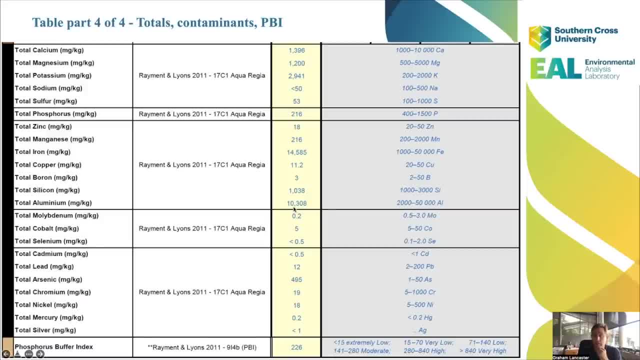 milligrams per kilogram, which is only one percent um. but yeah, people get very concerned about these numbers when they see them in a total form. it's only when you've got very acidic ph that you start getting these problems um. and then your molybdenum, cobalt, cadmium. this is looking at contamination. 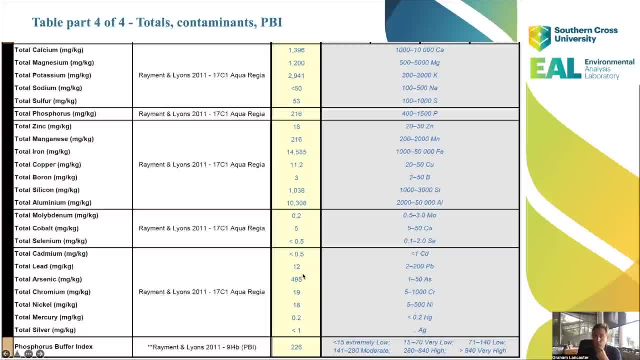 this soil. here is 595 milligrams per kilogram arsenic. it's contaminated very rarely do you find that naturally occurring. but naturally occurring you could have one to 50 milligrams per kilogram doesn't mean it's a problem. it should hopefully be heavily bound to the soil but this could be a serious problem for. 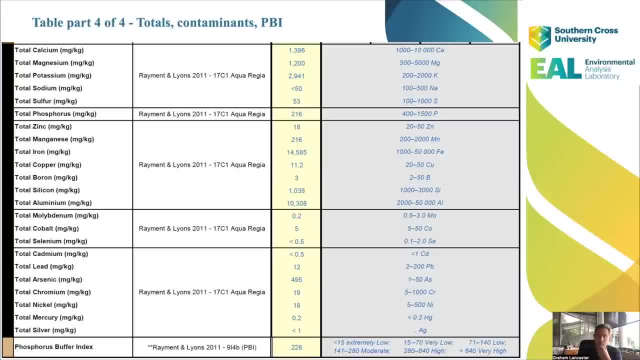 growing, especially organic crops. i've been to farms in england and europe where the lead content was 500 to a thousand milligrams per kilogram. if you're growing organic strawberries or organic crops in that sort of soil, it's inevitable you're going to get lead in your crops. that's a whole another. 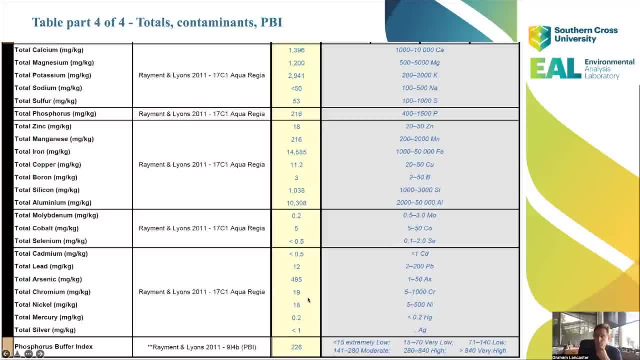 issue and the contamination of the issue. that must be addressed and can't be addressed just with soil biology. then you go through other elements and buffer index. you'll hear about these sort of phosphorus absorption capacity and all that. it's just the ability of the soil to bind. 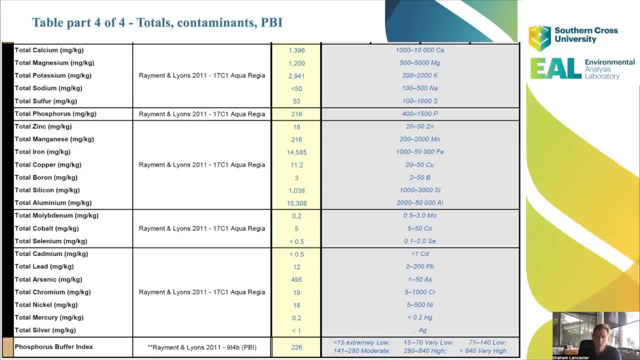 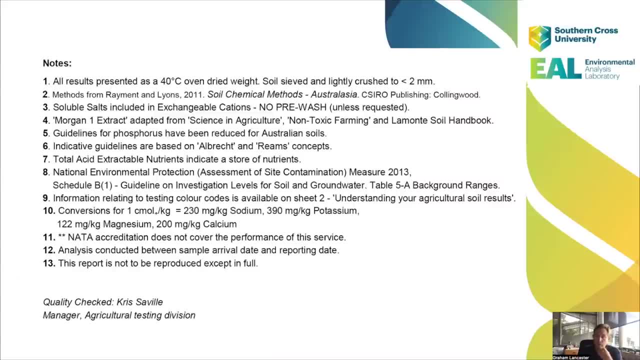 up your phosphorus, um- and we have some guidelines on that. i won't go to it into in many details to do today anyhow- um, we have some notes on our soil test to sort of explain what the results mean and and what the methods mean, and i think that's very important for labs to provide all this information. 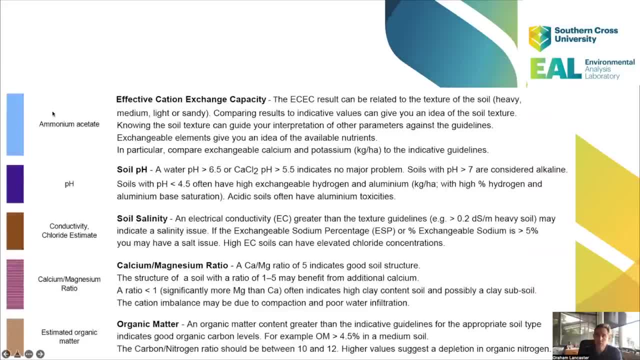 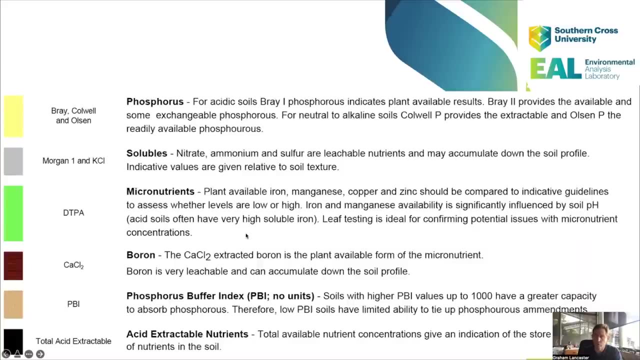 and then i color coded, or we color coded, each of our results up here so you can see there's greens and blues and that and that's where we just on our soil, test. we try to give some farmers some more information on what each of those means and a bit more interpretation of the results. so that's on our 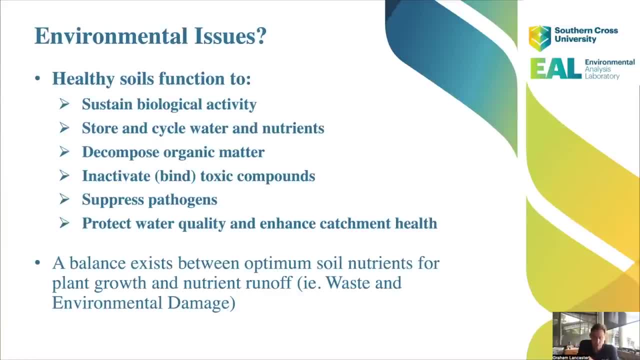 soil test as well. so we're trying to share this information so you don't have a dependence on agronomists. you really don't want to have be caught into the industry where you don't understand to some extent what results mean. i think it's important for traditional farmers or industrial. 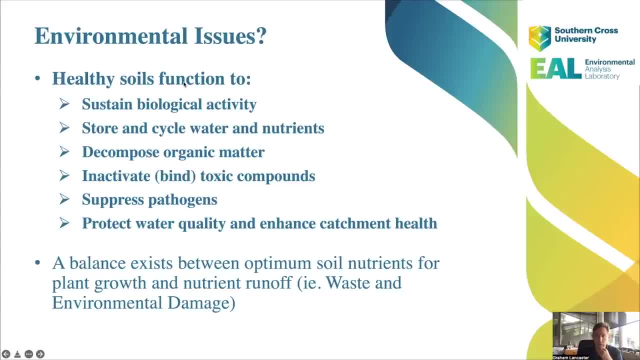 farmers, but ultra important for biological farmers, people that want to get away from the dependency on others, and really they say farming these days you've got to be a bit of everything. you've got to know it all: environmental issues, healthy soils function to sustain biological activities, store and cycle water and nutrients. 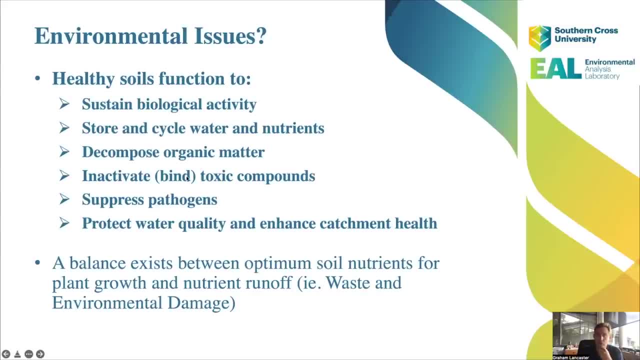 decompose organic matter, inactivate, bind toxic compounds. suppress pathogens. protect water quality, enhance catchment health. it's a big thing i got into when i got into doing environmental science degree that our rivers, our lakes, our oceans, especially our great barrier reef here in australia, really has poor water quality. that i'm sorry. it is attributed a lot to. 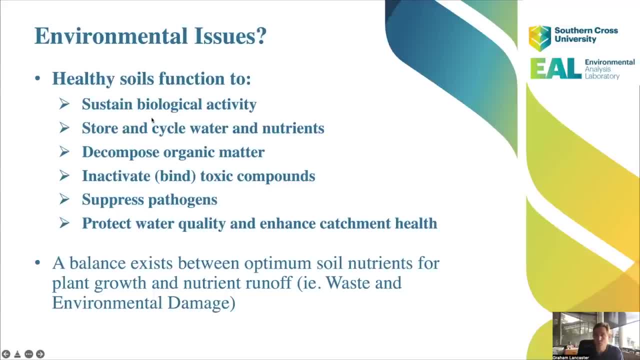 farming- putting excessive nutrients, excessive erosion, poor soil structure- so many issues there that that we need to address- and a balance exists between optimum soil nutrients for plant growth and nutrient runoff. we really don't want to see nutrient runoff or erosion and that's where we get the environmental damage that we. it's just a waste of money for a farmer if they're losing. 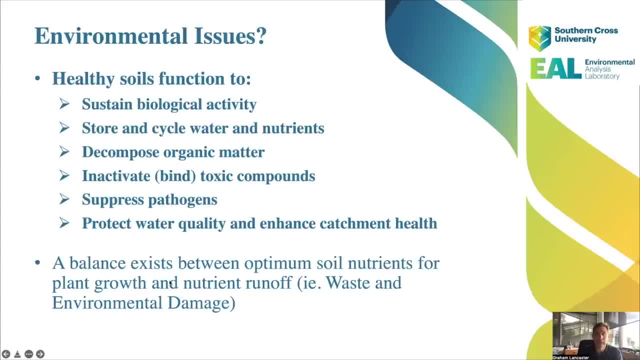 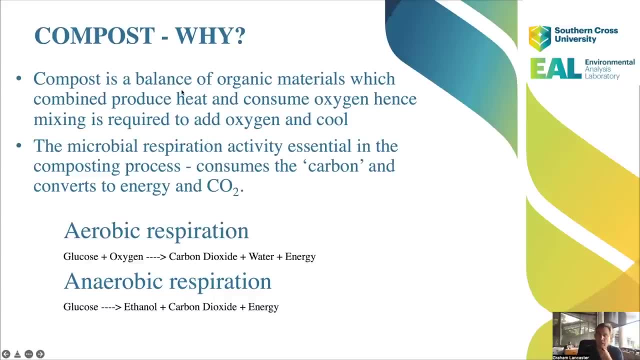 nutrients from their farm. they're just throwing their money down the drain. so compost why? obviously that's just the beauty of it. you know it's the little waste of energy we can't let you go. we go and feed the shit and, and you know, if i can't get some of that extra for myself to go, and i'm just 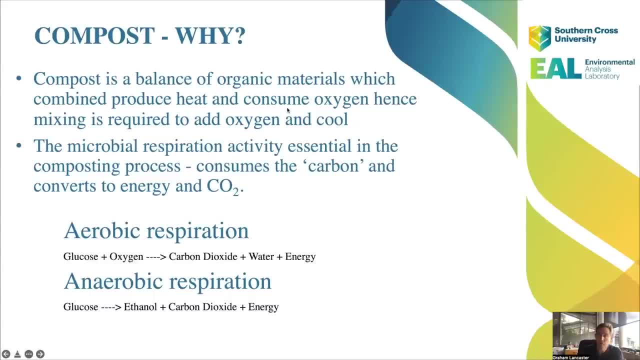 probably perspiring to look at it, and at least it wasn't a big deal for me. so, um, so our last few videos are going to be about this. this is pretty much a very short one, so i hope you have a good time watching um, and i do think that there's a lot of good things about us. i hope you make a big difference and i 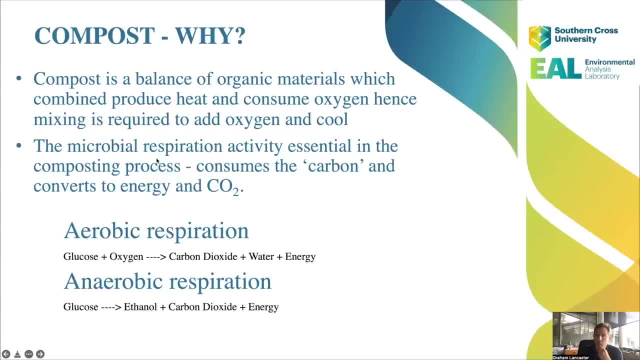 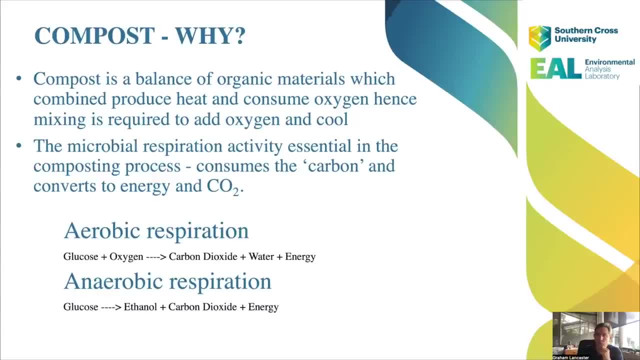 a worry for people that they get concerned about this, but it's such a natural process because it converts the carbon into energy and CO2.. Now we say about CO2 being a problem in the atmosphere. A lot of our losses in traditional farming is from the stir up, the 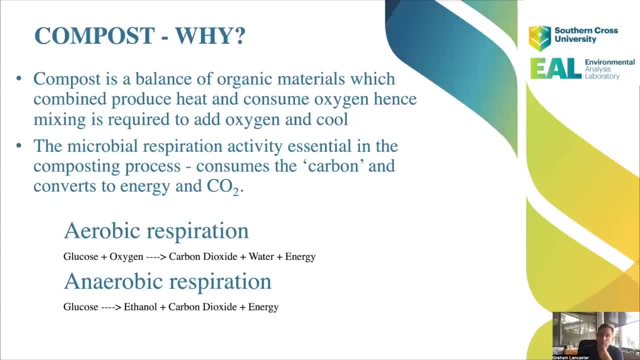 cultivation of soils, excessive cultivation of soils, which aerates the soils, which increases the microbial activity, which consumes the carbon in soil and releases CO2.. So in traditional farming, where we've just liked to see beautiful pastures and soils that are really finely. 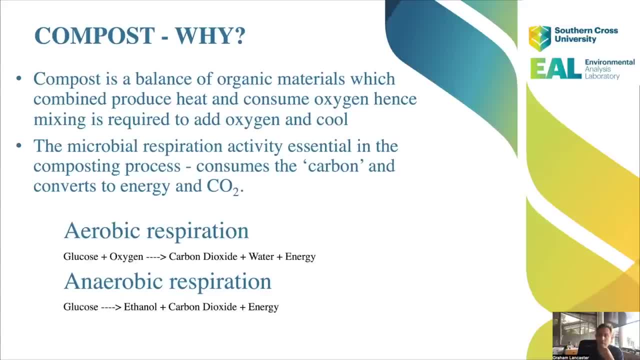 cultivated 00.01.190,00.01.190 By all different cultivation techniques. this has produced a lot of the loss of our carbon in our soil. So now we have direct drilling, reduced cultivation and areas which doesn't burn away this soil from the carbon from the soil. But look, aerobic respiration is glucose. 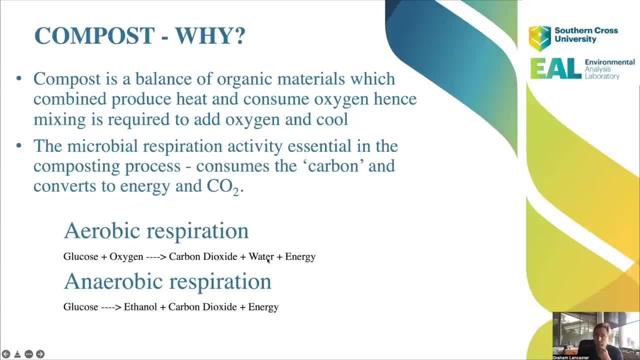 plus oxygen gives carbon dioxide, plus water, plus energy. That glucose is your carbon in your process- 00.01.190,00.01.190. And aerobic respiration is another form of making compost. You've got to know what you're doing, because it does produce ethanol, which can evaporate away carbon dioxide and energy. 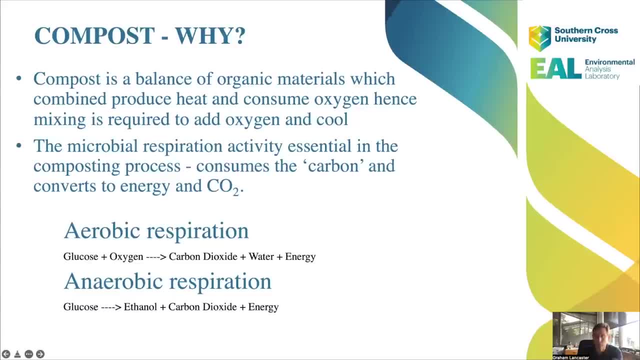 So this process is just such a natural process of decomposition of carbon in the soil or taking organic matter in the right balance of carbon nitrogen ratio to make a really healthy, nutrient rich additive for farming- 00.01.190,00.01.190. 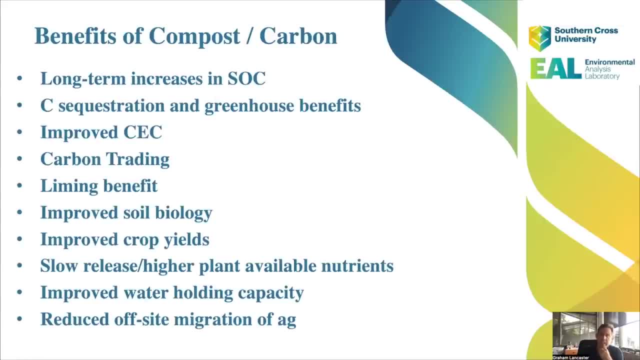 And, as I say, it's a natural process- 00.01.190,00.01.190. So the benefits of carbon in compost is similar to the benefits of carbon in your soil. You really want to see a long term increases in soil organic carbon, And that's what we sell. 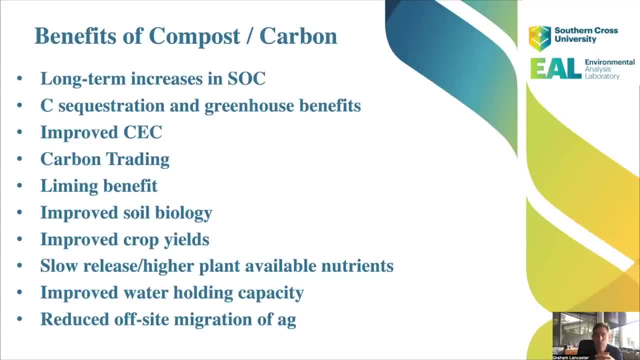 our carbon credits on And we want to see that right down the soil profile to a meter if possible. 00.01.190,00.01.190. We want to see carbon sequestration, which is binding up all this carbon in the soil. 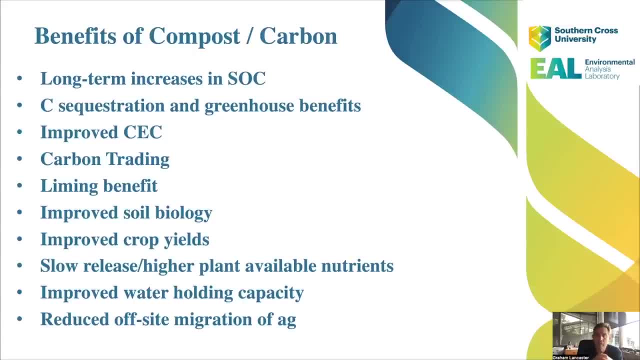 which obviously greenhouse benefits. 00.01.190,00.01.190. If we can bind that CO2 into our soils and bind it in there in carbon, it's a benefit for farming and for the environment. 00.01.190,00.01.190. 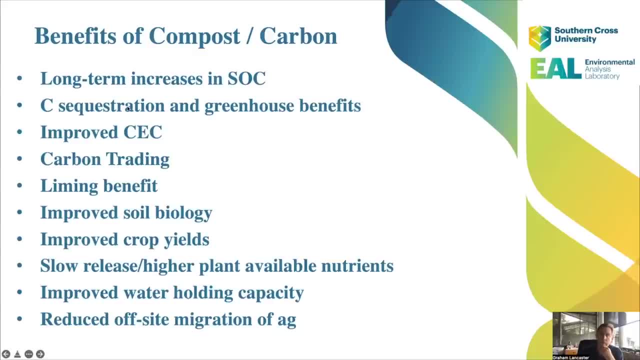 Improved cation exchange capacity. If we can build up that carbon in the soil, we will build up that cation exchange capacity or the ability to store cations. 00.01.190,00.01.190. Carbon trading- hopefully a big money source for farmers in the future and even now. 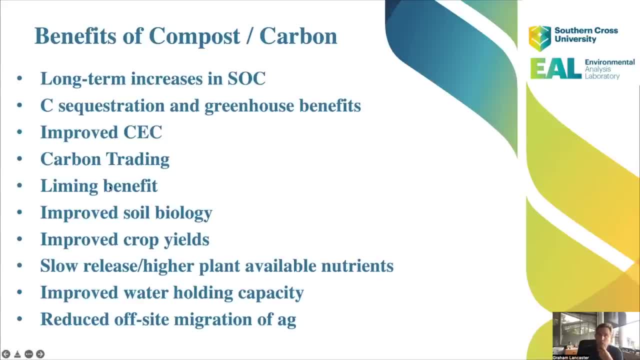 00.01.190,00.01.190 Liming benefit. like I mentioned, building up your compost and your carbon in your soil. 00.01.190,00.01.190. Carbon in your soil often neutralises your soil. 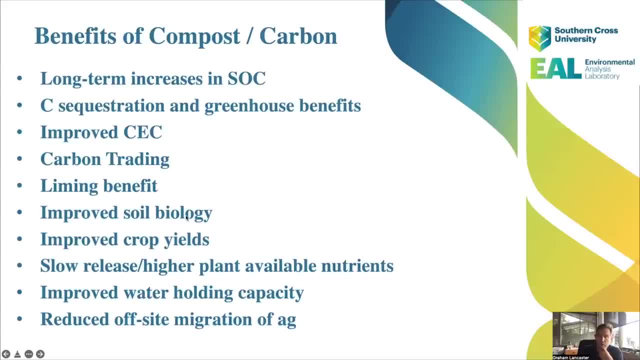 00.01.190,00.01.190. Improved soil biology. Huge aspect of building up your carbon to build up your soil biology. Improved crop yields very achievable, So slow release. higher plant available nutrients- 00.01.190,00.01.190. 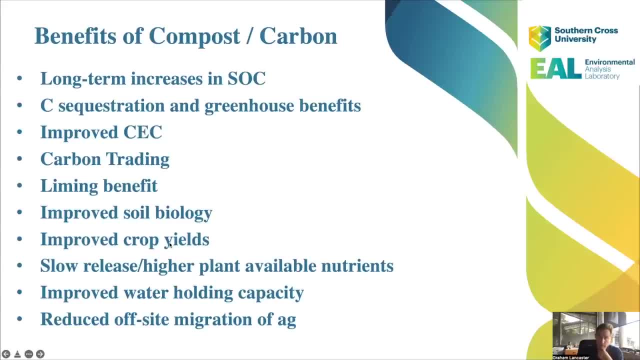 And this is which is with increasing cation exchange capacity builds up this increasing stored to some extent and release of nutrients. 00.01.190,00.01.190- Improved water holding capacity. As I started my presentation, I was talking about this. 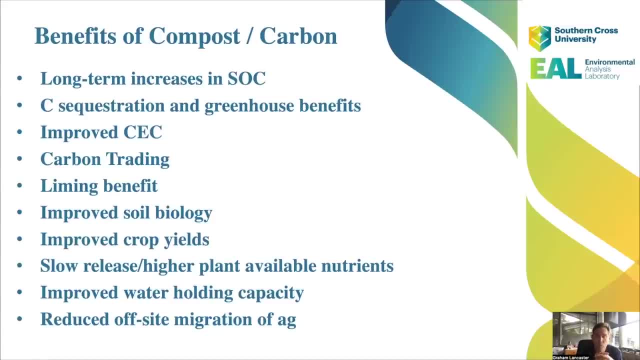 about floods: 00.01.190,00.01.190. The opposite of floods is droughts, and they do occur and will keep on occurring around the world. 00.01.190,00.01.190. And we really want to be able to store as much water in our soils, and that's where. 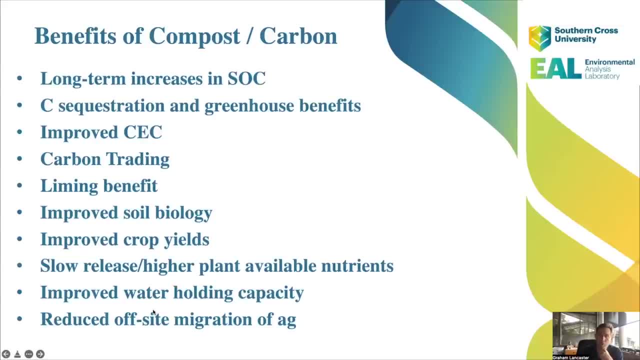 the carbon and compost can help. 00.01.190,00.01.190. Reduced offsite migration of ag chemicals or metals or contaminants. 00.01.190,00.01.190. We really want to bind them up with the carbon. 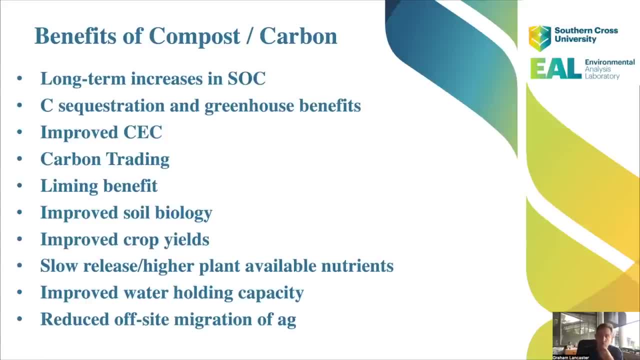 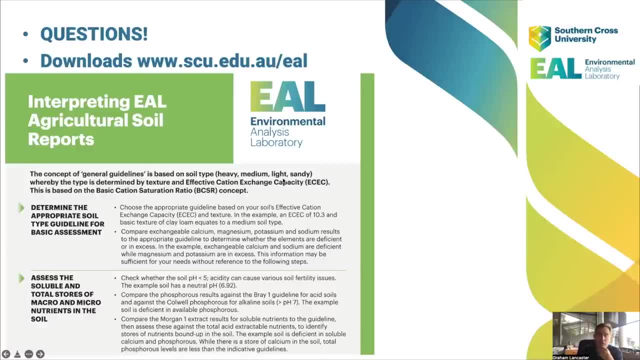 We don't want to see them going into the environment or into our food systems. 00.01.190,00.01.190. 00.01.190,00.01.190. So really, that's a very brief overview of soil chemistry, soil biology and the physical. 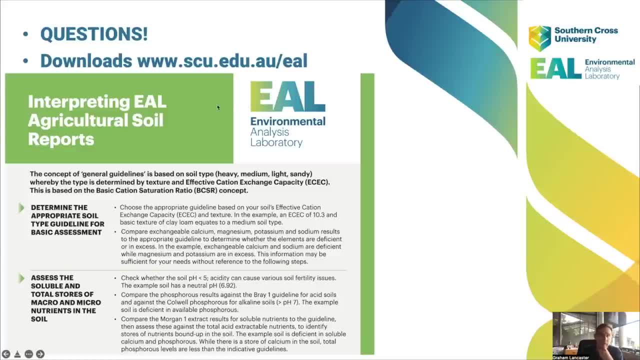 structure of our soils and nutrient cycling In our download on EAL. we have a lot of free downloads there. I've got a bit of interpreting EAL- agricultural soil reports. This applies to any soil report, It's not just EALs, but I've tried to make it quite simple so you can get some understanding. 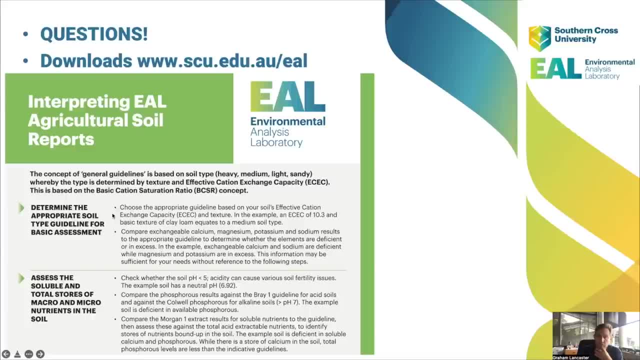 And it just has a different descriptive here: 00.01.190,00.01.190- 00.01.190,00.01.190. So you can use that to determine the appropriate soil type, which I've mentioned quite detailed. 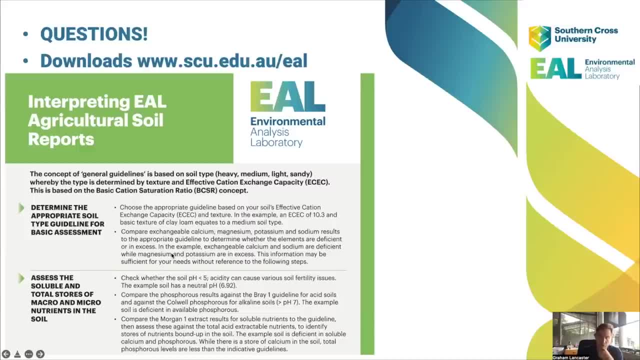 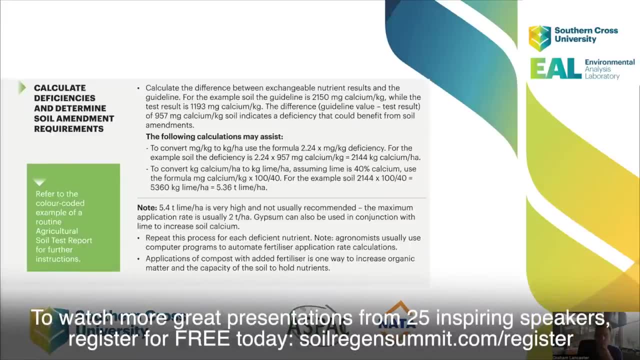 And basing back to those soil results I was just talking about, And I won't go through this in this talk, but there's two pages there, or one page, but I've got it over two slides here to really go through an example. and, yeah, see how you. 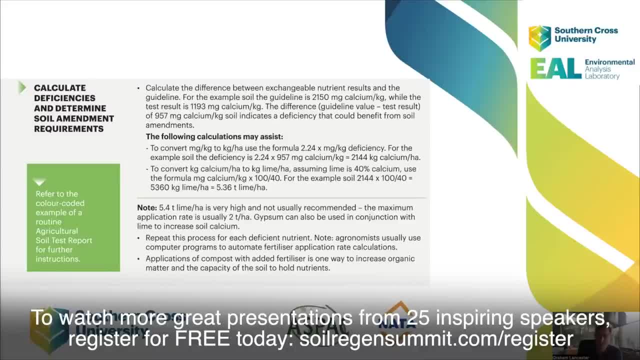 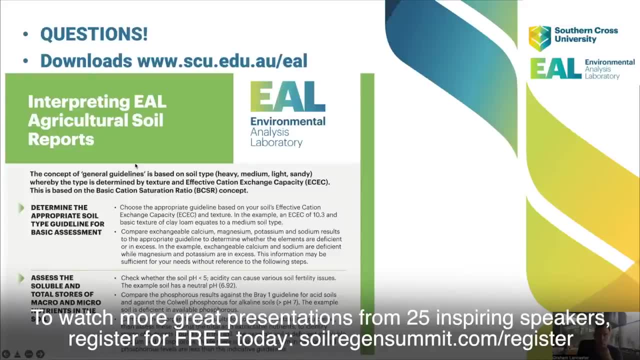 can interpret your results to really help your biological farming journey. So I'll wish you well on your journey. It's not a quick journey, but it is a worthwhile journey. 00.01.190,00.01.190. So thank you for your time today and enjoy the symposium. 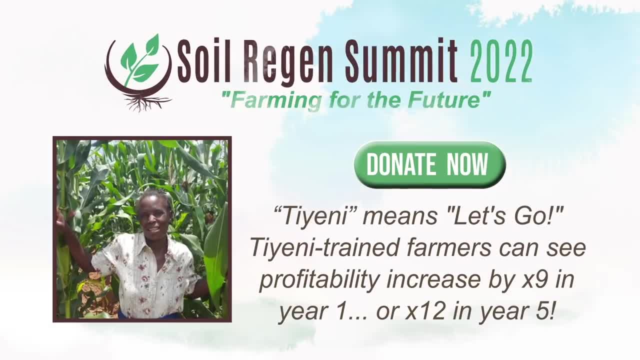 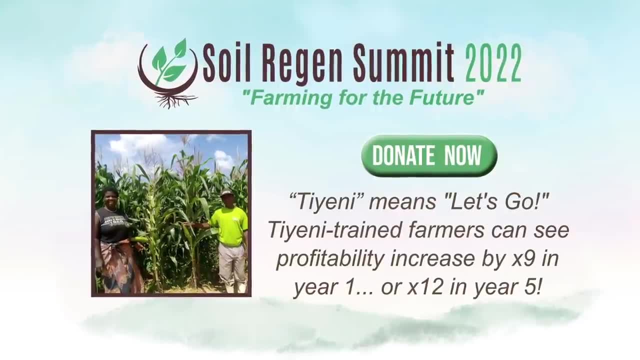 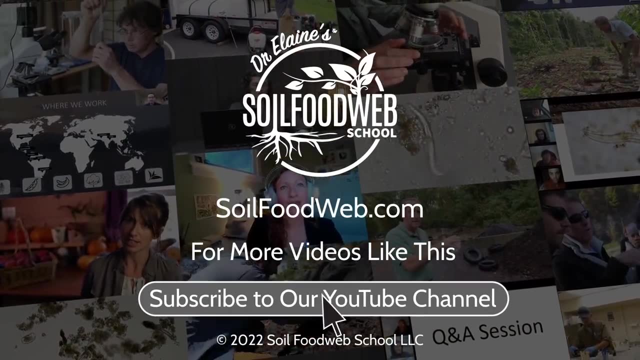 All right, thank you. T&E means let's go. T&E- trained farmers can see profitability increase by nine times in year one, or 12 times in year five. For more videos like this, subscribe to our YouTube channel. 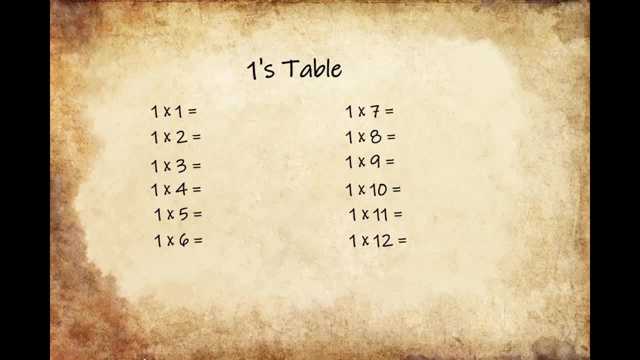 Today we're going to be looking at multiplication tables from 1 through 12.. 1 times 1 is 1.. 1 times 2 is 2.. 1 times 3 is 3.. 1 times 4 is 4.. 1 times 5 is 5.. 1 times 6 is 6.. 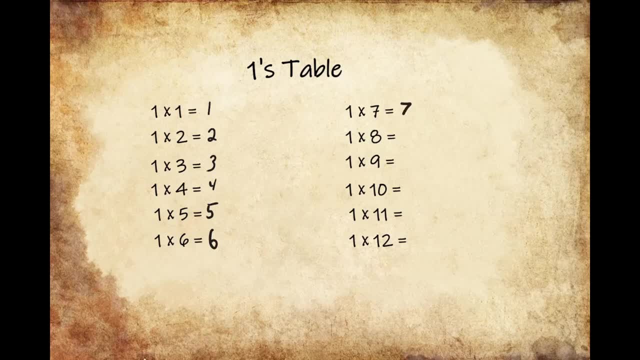 1 times 7 is 7.. 1 times 8 is 8.. 1 times 9 is 9.. 1 times 10 is 10.. 1 times 11 is 11.. 1 times 12 is 12.. 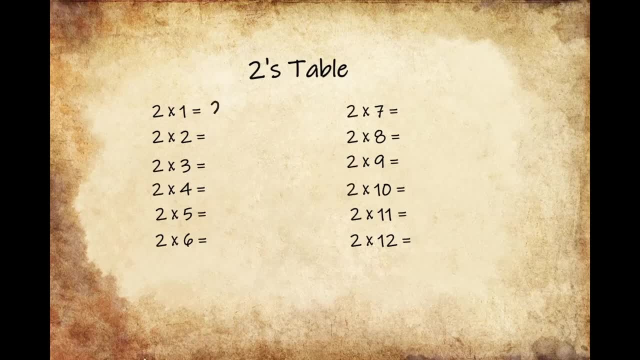 Looking at the twos table: 2 times 1 is 2.. 2 times 2 is 4.. 2 times 3 is 6.. 2 times 4 is 8.. 2 times 5.. 2 times 6 is 12.. 2 times 7 is 14.. 2 times 8 is 16.. 2 times 9 is 18.. 2 times 10 is 20.. 2 times 11 is 22..